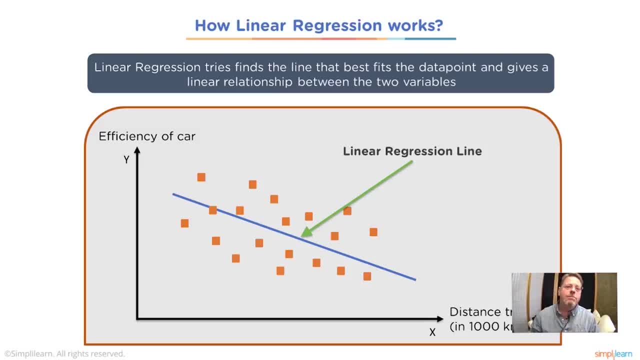 see this nice straight line drawn through there, And when you talk about multiple variables, all you're doing is putting this: instead of a line it now becomes a plane. It gets a little complicated with multiple variables, but they all come down to this linear kind of drawing a line. 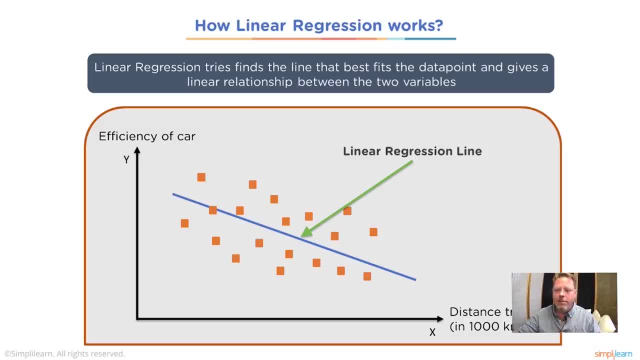 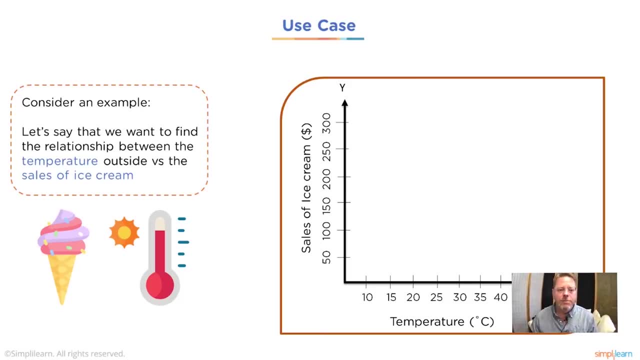 through your data and finding what fits the data the best. And so we can consider an example. Let's say that we want to find the relationship between the temperature outside versus the sales of ice cream, And so we start looking at that. We're looking at how many ice cream cones we're selling. 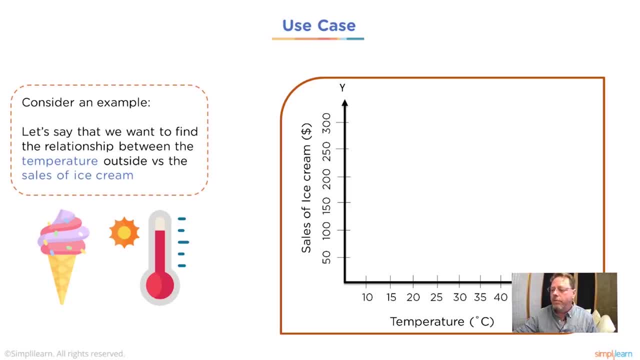 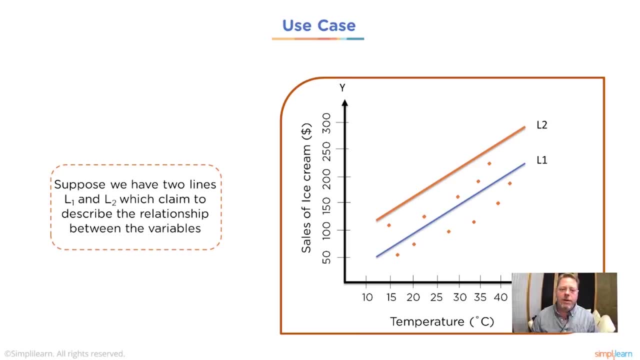 or how much money. we sold an ice cream And we're looking at how warm it is outside, which would hopefully draw a lot of people into the ice cream store, And suppose we have two lines. We're going to draw L1 and L2.. And we're going to kind of guess which one we think is the best fit. 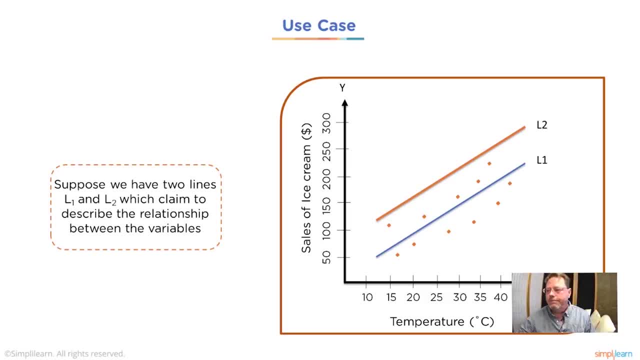 And which claim to describe the relationship between the variables. And so first we find the square of the distance between the line L1 and each data point and add them all and find the mean distance. And I want you to think about that when we square something, If it's a negative or positive. 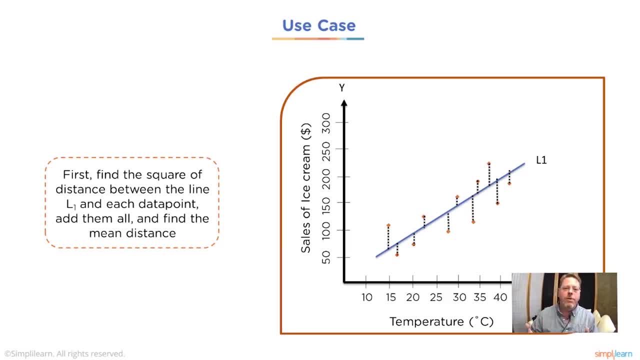 number no longer matters, because a minus two squared is four. two squared is four. So we're removing what side of the line it's on and we're just looking for the error, In this case the mean distance of each of the little dotted lines. you see here This way of calculating the square of. 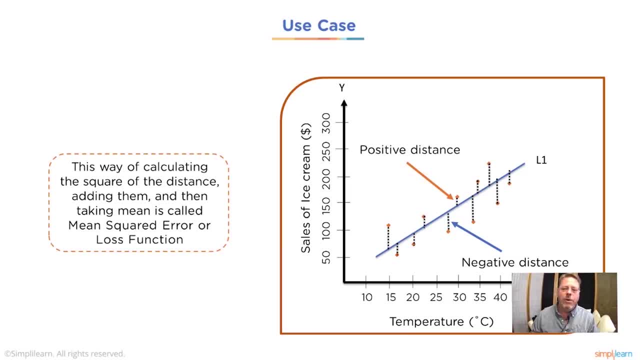 the distance. adding them and then taking the mean is called mean square, error or loss function. And we talk about loss. How far off are we? That's what we're really talking about. What did we miss? And we have a positive distance and a negative distance And, of course, when we square it, it is neither It just. 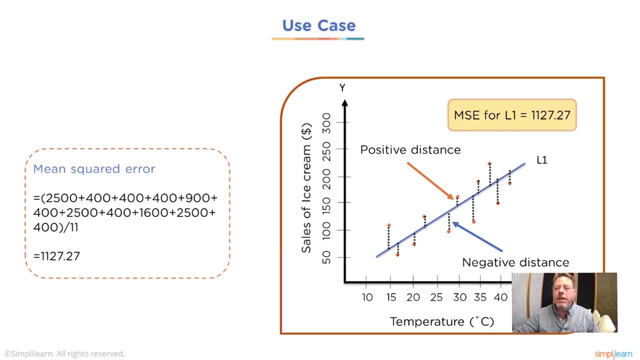 becomes a positive error. And so we take the mean square error and a lot of times you'll see it referred to as MSE. If I look in a code and I'm going through my Python code and I see MSE, I know that's the mean squared error And we take all the dotted lines and we calculate this error, We add: 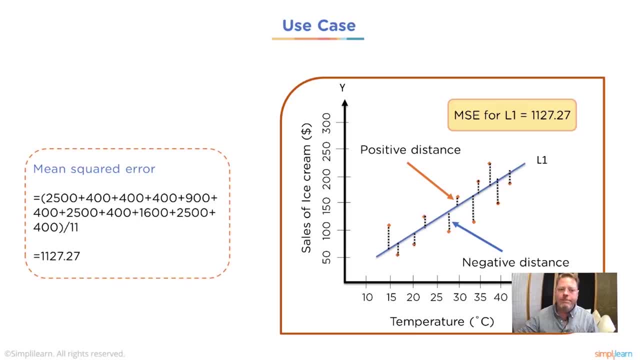 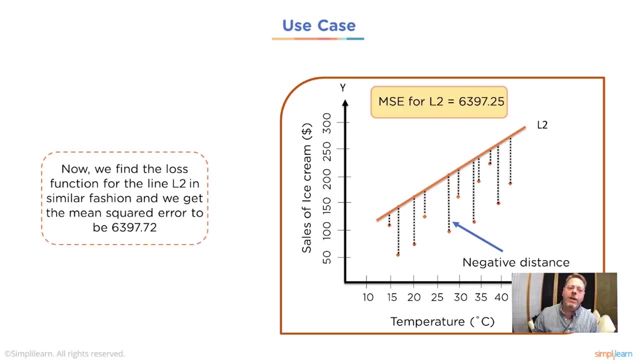 them all together and then we average it or find the means, And in this case they ran a demo on this and it was 1127.27 for our L1 line. Now we find the loss function for line L2 in a similar fashion and we get the mean square error to be 6397.. And it's computed the same way. So maybe you put. 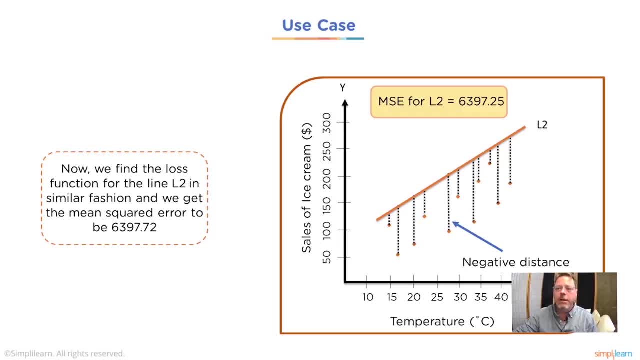 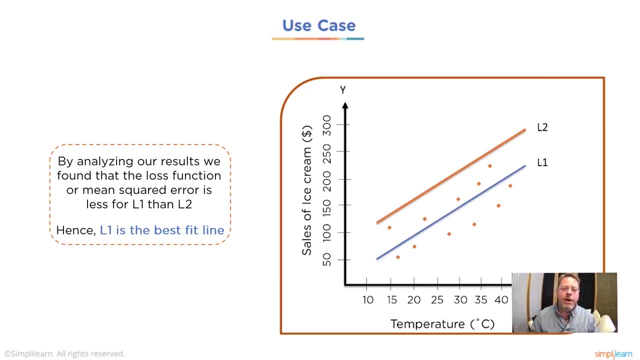 this line just way outside the data range, and this is the error you get. By analyzing our results, we find that the error is less for L1 than L2. Hence L1 is the best fit line. This process describes a lot of. 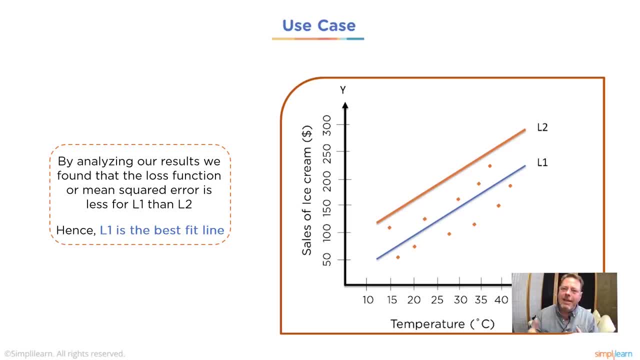 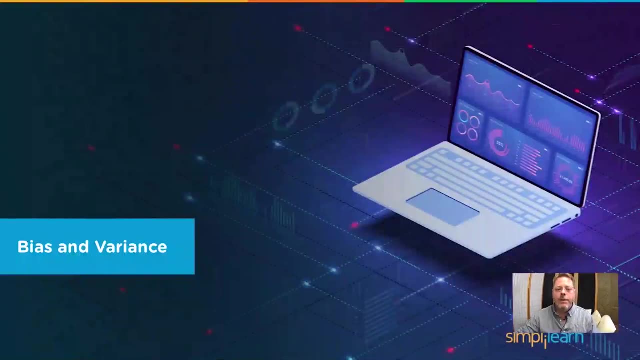 machine learning processes. We're going to keep guessing and get as close as we can to find the right answer. We have to have some way to calculate this and figure out which one is the best, And the mean square error is one of the better fits for doing this and most commonly used. We really want to talk about. 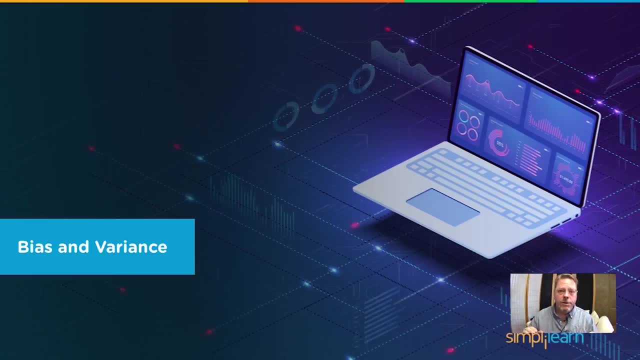 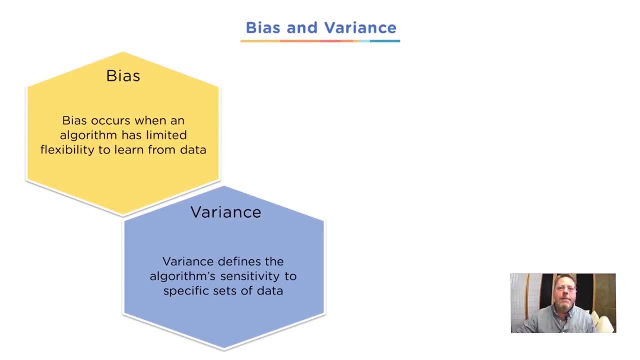 bias and variance- Very important terms to know in machine learning and with linear regression. So bias: Bias occurs when an algorithm has limited flexibility to learn from data. Variance defines the algorithm's sensitivity to specific sets of data. Let's start with bias and variance. You can see here we have the two different. 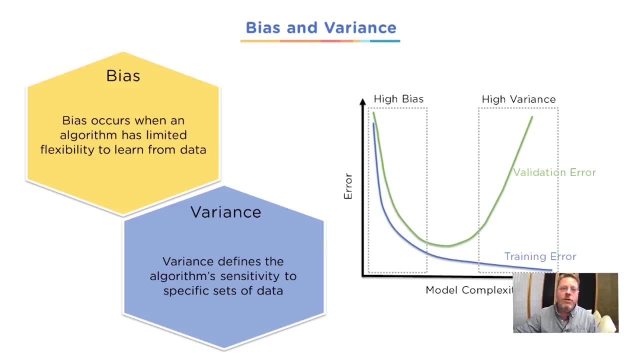 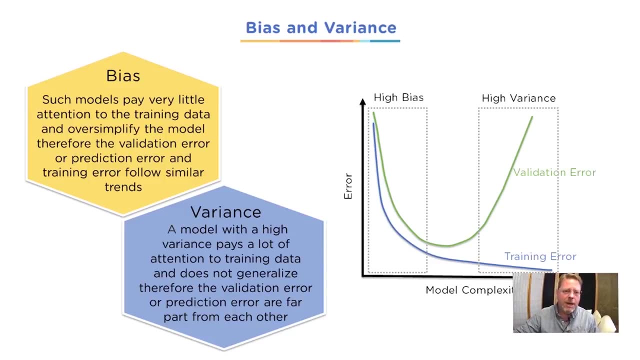 setups. Bias, you can think, is very generalized, where variance is very specific, And so we talk about bias. Such models pay very little attention to the training data and oversimplify the model. Therefore the validation error or prediction error and training error. 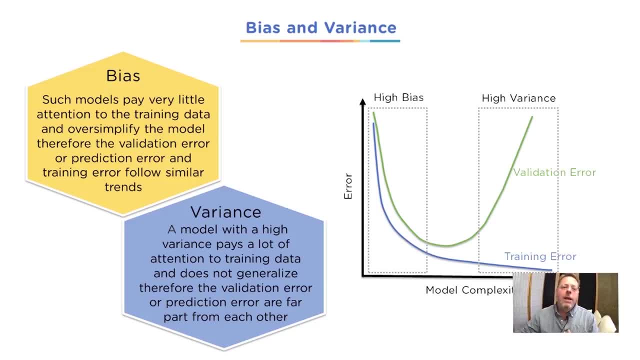 follow similar trends And with bias. if you oversimplify it so much, you're going to miss your local. if you have a really good fit, you're going to miss it. You're going to just kind of guess what the average is and that's what your answer is going to be. 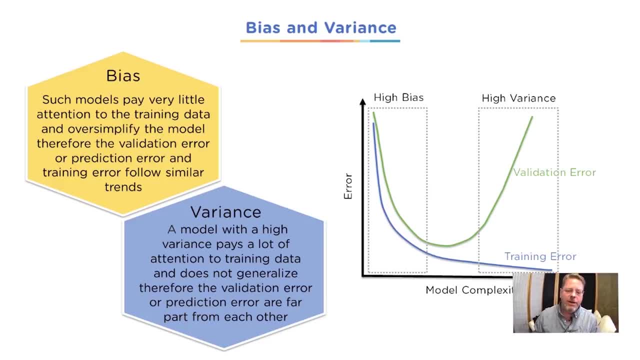 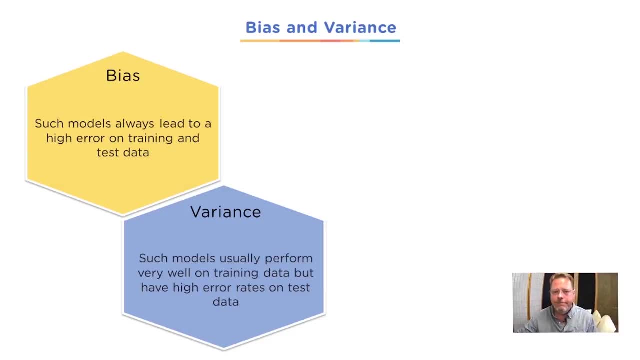 With variance. a model with a high variance pays a lot of attention to training data and does not generalize. Therefore, the validation error or prediction error are far apart from each other. Such models always lead to a high error on training and test data, as a bias does. Where variance, such models usually perform very well on 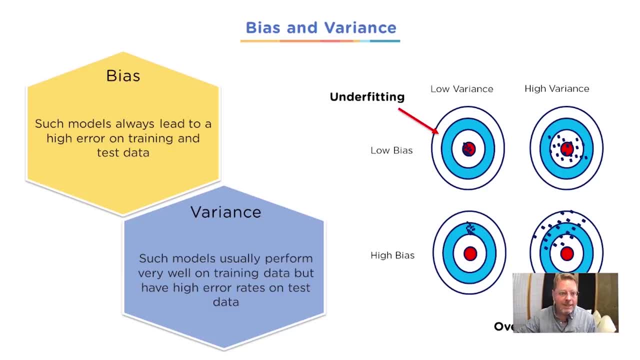 training data but have high error rates on test data. And I want you to think about this: When we're talking about a bias, the error is going to be high, both when you're training it and you're testing it. Why? Because we're just kind of getting an average. We're not really fitting it close. 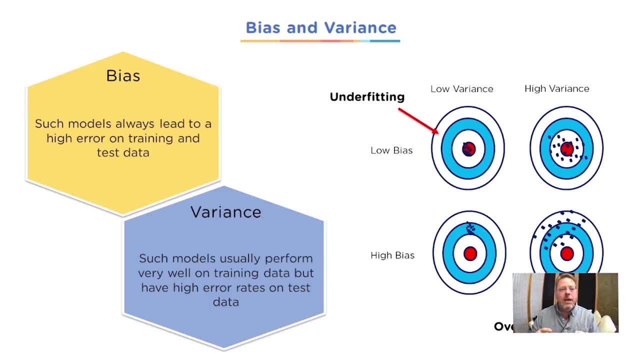 With variance. we're fitting it so close that the test data does really good. It's going to nail it every time. If you're doing categorical testing, that's a car, that's a truck, that's a bicycle, But with variance. 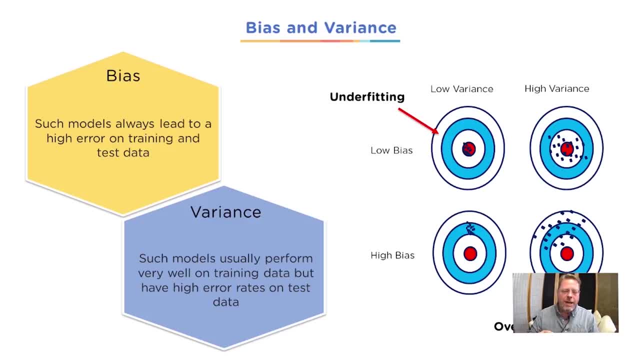 suddenly, a truck has to have certain features and it might have to be red because you had so many red pictures. So if it's an 18-wheeler, it has to be red. If it's blue, then it has to be a bicycle. 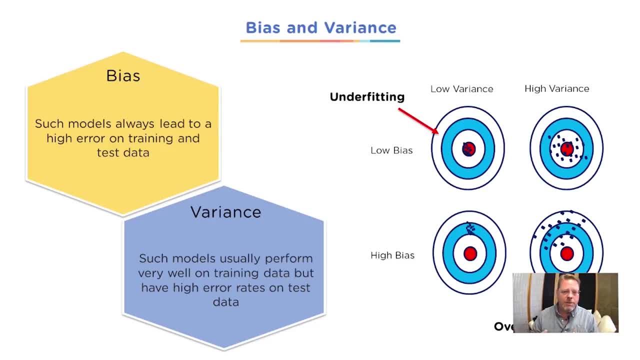 That's the kind of variance we're talking about, where it picks up on something and it cannot get the right answer unless it gets a very specific data. And we see that so that, as you're testing it in your models and you programmed it, you got to look for. 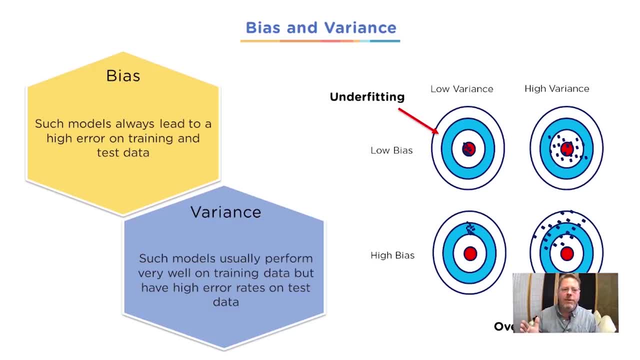 how I trained it. what is coming out and if it's not looking good on either bias or if it's not looking good on the training or on the test data, then you're bias in your data. If it really looks good on the training data, 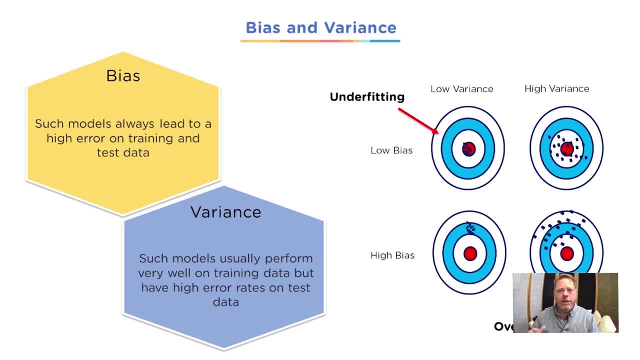 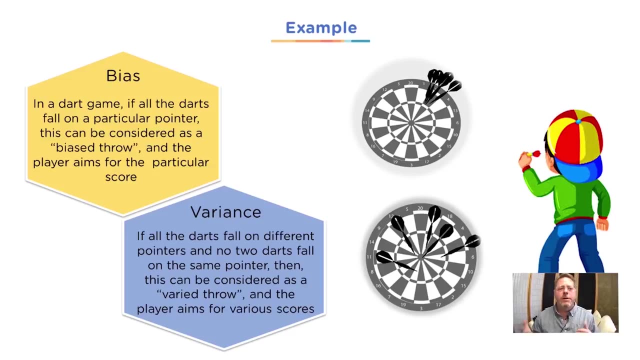 then that's going to be your variance. You've overfitted the data, And those are very important things to know when you are building your models in regression of any kind or any kind of setup for predicting. So in dart games, if all the data fall on a particular pointer, 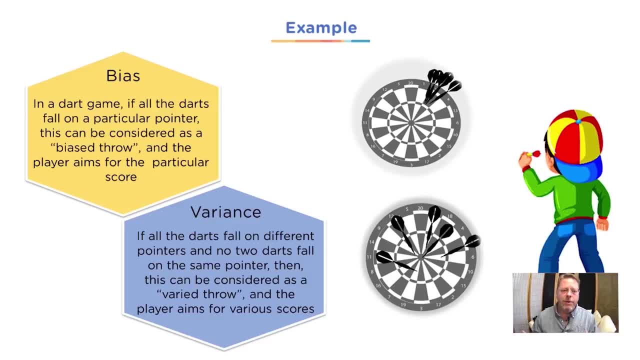 this can be considered as a biased throw and the player aims for the particular score For variance. if all the darts fall on different pointers and no two darts fall on the same pointer, then this can be considered as a varied throw and the player aims for various scores. 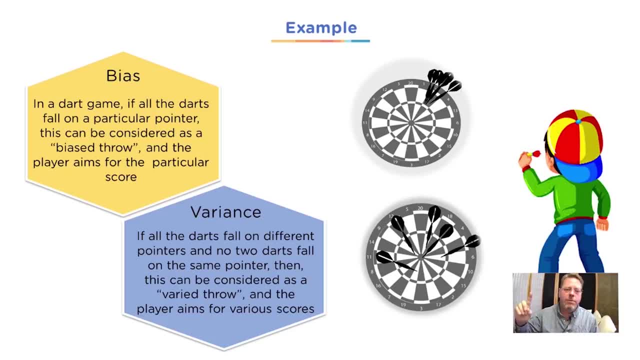 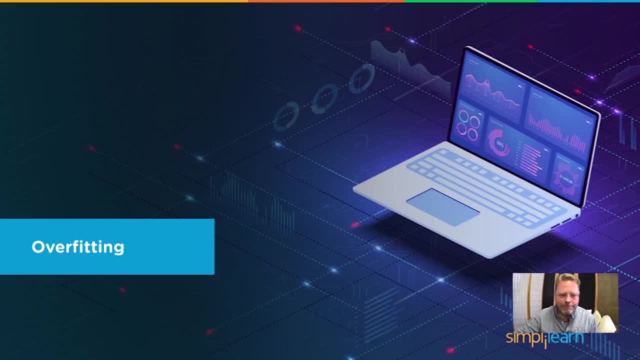 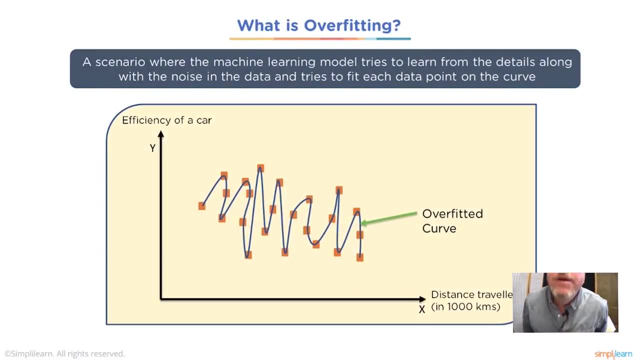 Again, the bias sums everything up in one point, kind of averages it together, where the variance really looks for the individual predictions coming out. So let's go ahead and talk about overfitting. When we talk about overfitting, it's a scenario where the machine learning model tries to learn from the details, along with the noise. 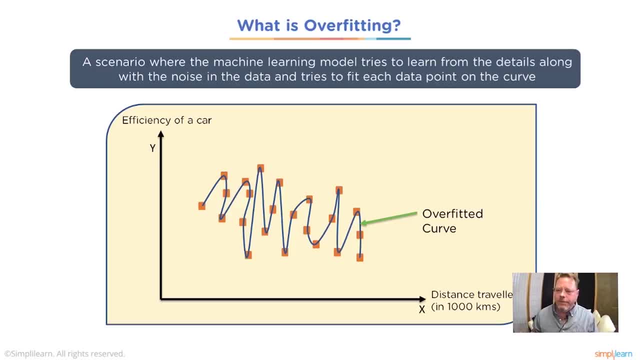 and the data tries to fit each data point on the curve. You can see that if you plug in your coordinates you're just going to get the whatever is fitted, every point on the data stream. There's no average, There's no two points that might have the 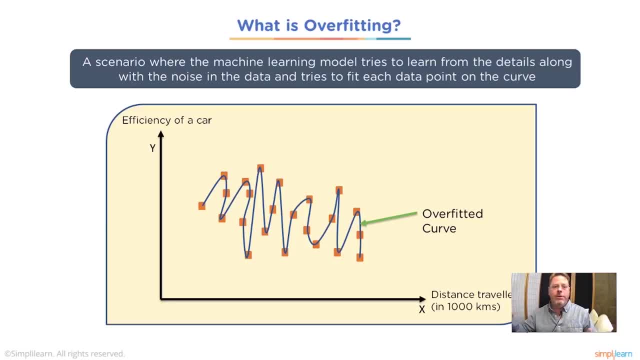 you know two different answers, because if the wind blows a certain way and the efficiency of your car maybe you have a headwind, So your car might alter how efficient it is as it goes, And so there's going to be this variance on here. 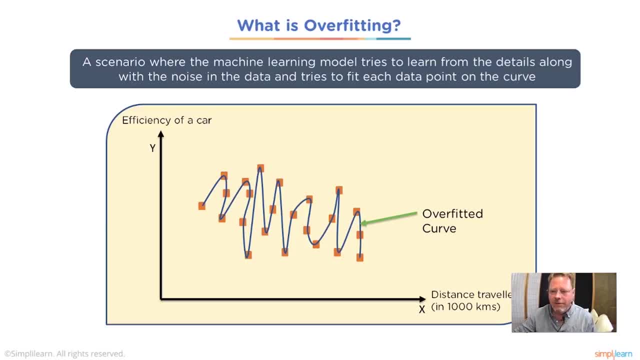 And this says no, you can't have any variance with you know, this is going to be exactly this. It can't be any. you can't be the same speed or the same car and have a slightly different efficiency. So, as the model has very less flexibility, 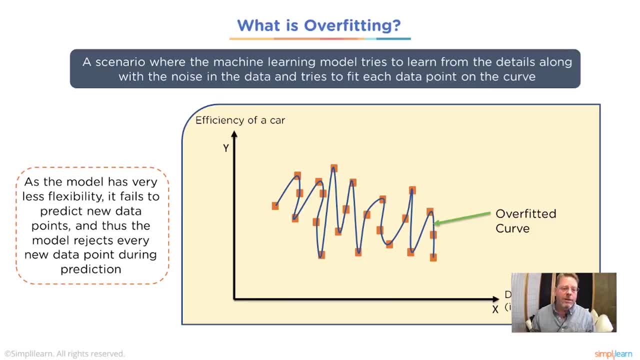 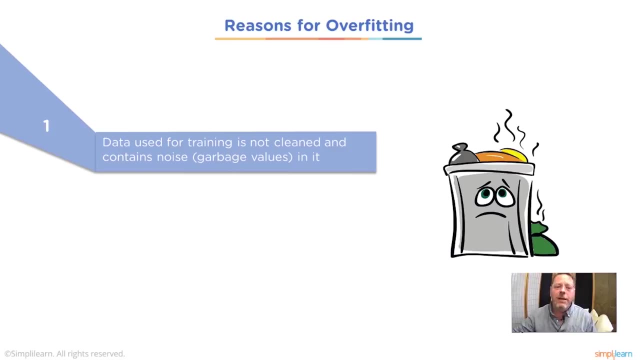 it fails to predict new data points, And thus the model rejects every new data point during the prediction, So you'll get like a really high error on here. And so reasons for overfitting. Data used for training is not cleaned and contains noise. 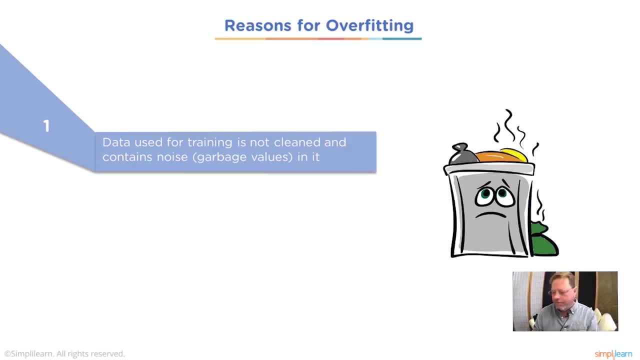 garbage values in it. You can spend so much time cleaning your data And it's so important. It's so important that if you have, if you have, some kind of something wrong with the data coming in, it needs to be addressed, Whether it's a source of the data. 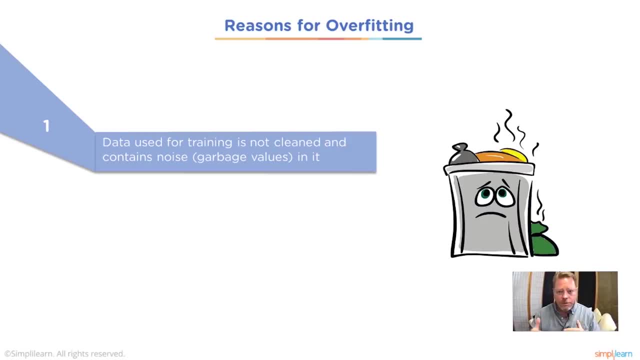 maybe they use in medical different measuring tools. So you now have to adjust for data that came in from hospital A versus hospital B or even off of machine A and machine B. that's testing something And those, those numbers are coming in wrong. 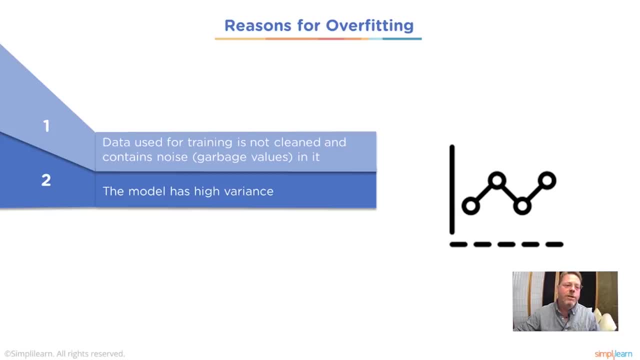 The model has a high variance. Again, wind is a good example. I was talking about that with the car. You may have a hundred tests, but because the wind's blowing, it's all over the place. Size of training data used is not enough. 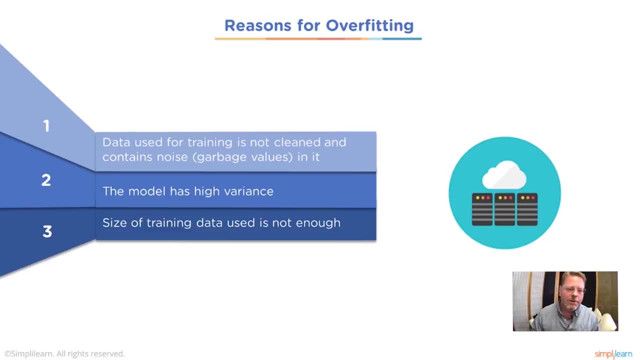 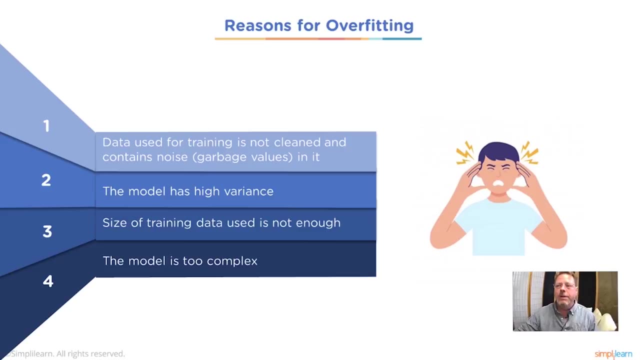 So a small amount of data is going to also cause this problem. You only have a few points and you try to plot everything. The model is too complex. This comes up a lot. We put too many pieces together, and how they interact can't even be tracked. 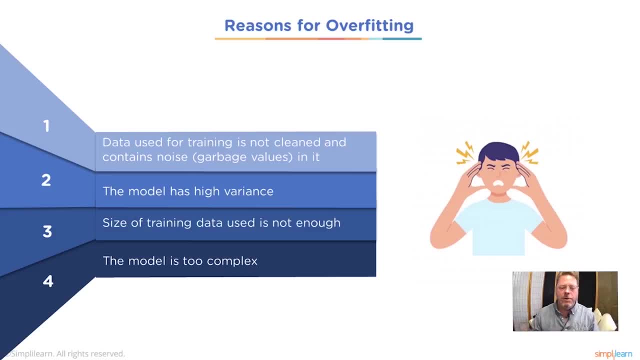 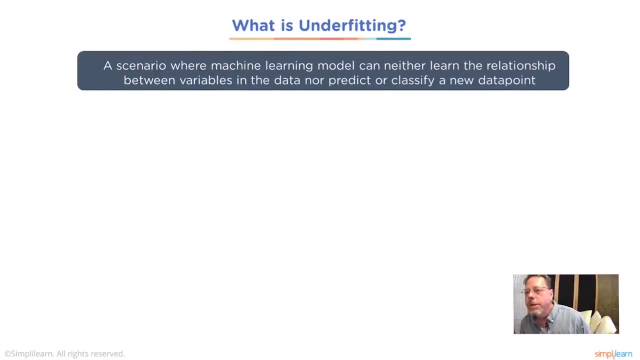 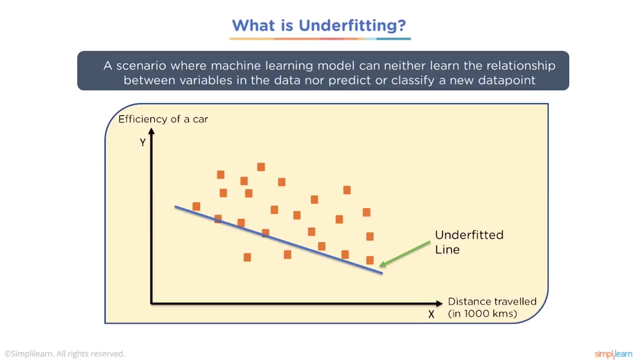 And so you have to go back, break it up and find out actually what correlates and what doesn't. So what is underfitting A scenario where machine learning models can either learn the relationship between the data points, nor predict or classify a new data point? 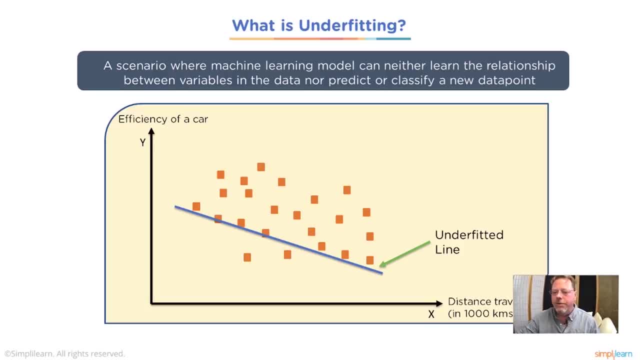 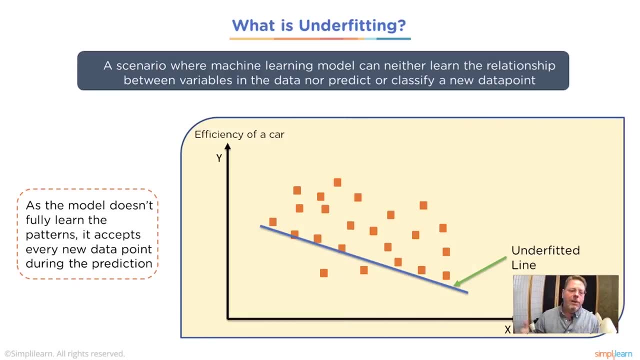 And you can see, here we have our efficiency of our car and our line drawn and it's just going to be way off for both the training and the predicting data. As the model doesn't fully learn the patterns, it accepts every new data point during the prediction. 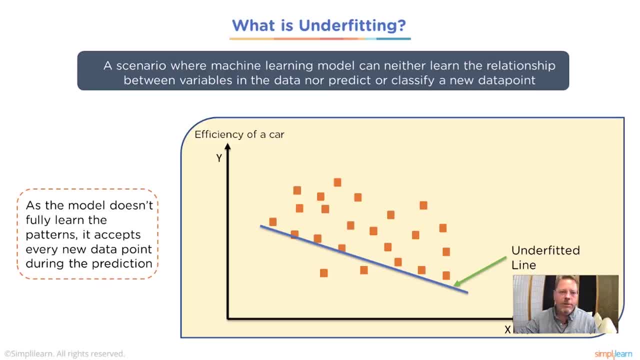 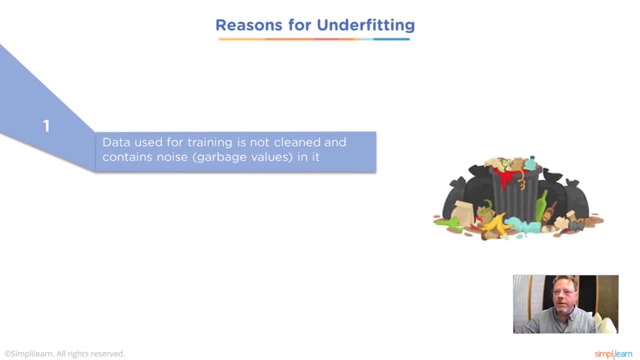 So, instead of looking for a general pattern, uh, just kind of accept everything. Data used for training is not cleaned and contains noise, garbage and values- Again underfitting and overfitting same issue. You got to clean your data. 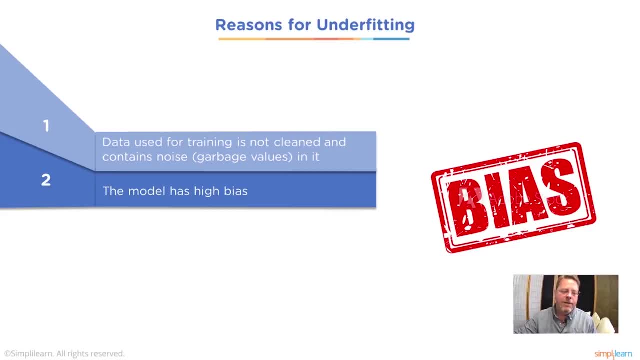 The model has a high bias. Uh, we've seen this in all kinds of things, from- uh, the most common is the driving cars- to facial identification or whatever it is. The model itself, when they build it, might have a bias towards one thing. 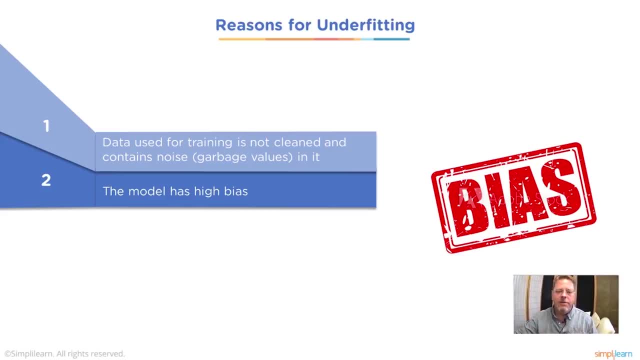 And this would be an underfitted model- would have that bias because it's averaged it out. So if you have, uh, five people from India and 10 people from um Africa and 20 people from the US, you created a bias. 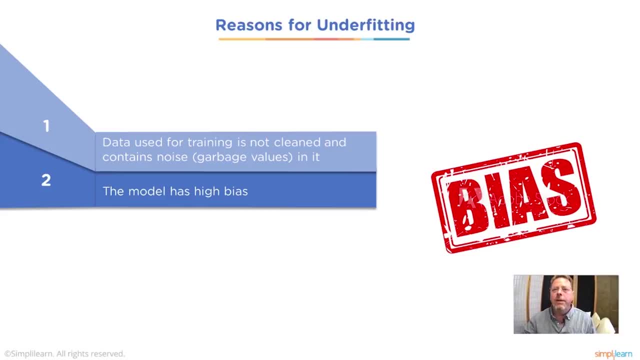 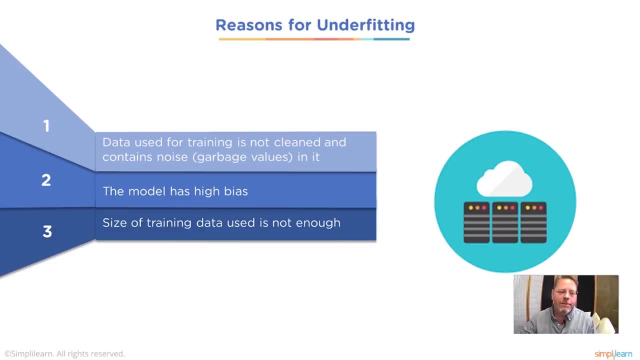 uh, because it's looking at the 20 people and you only have a small amount of data to work with. Size of training: data used is not enough. Uh, that goes with the size I was just talking about. So we have a model with a high bias. 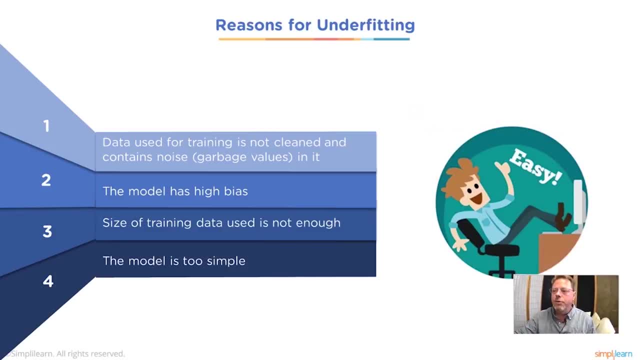 We have size of training data used. It's not enough. The model is too simple. Again, this is one straight line through all the data when it needs as a slight shift to it for other reasons. So what is a good fit? Uh? 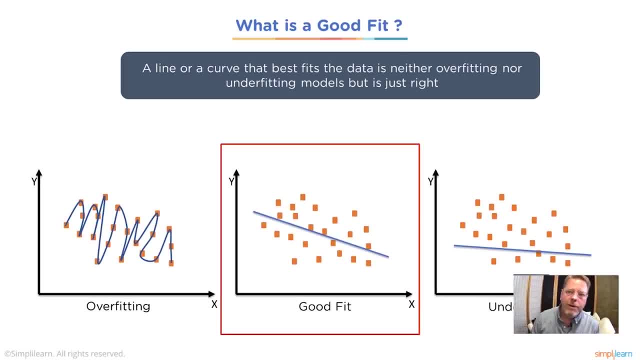 a linear curve that best fits the data, is neither overfitting or underfitting models, but is just right. And of course we have the nice examples here where we have overfitting lines going up and down. Every point is trying to be included. 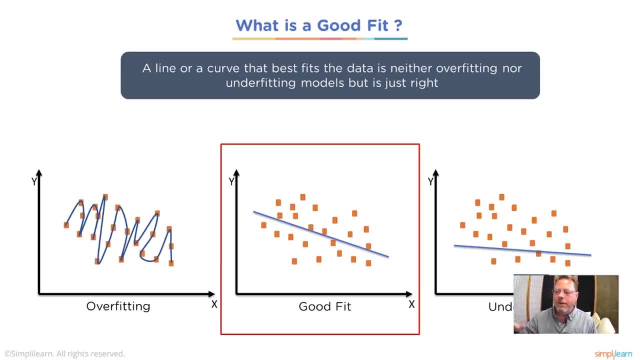 included underfitting. Uh, the line really is off from where the data is, And then a good fit is got to get rid of that, minimize that. um error coming through Regularization is taking the guesswork out. You're looking at this graph and you're going. 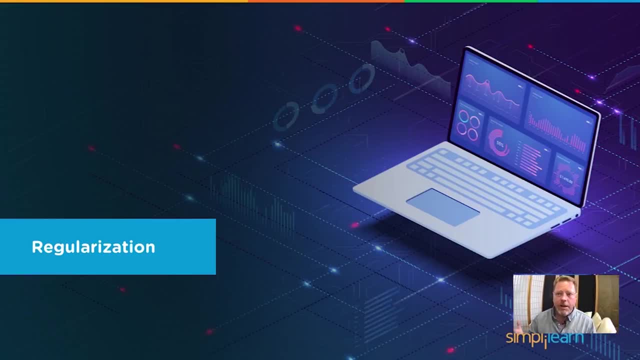 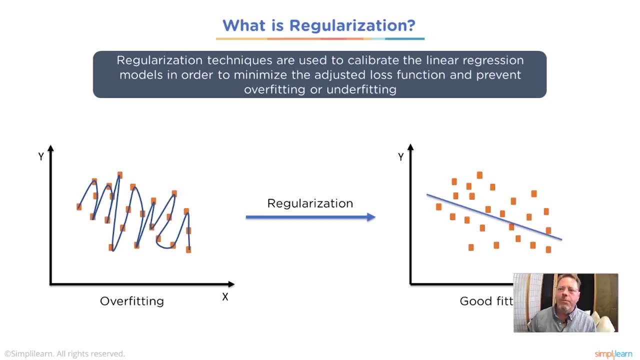 Oh, which one? is that really overfit or is that under fit? That was pretty hard to tell. So we talk about regularization. Regularization techniques are used to calibrate the linear regression models and to minimize the adjusted loss function and prevent overfitting or underfitting. 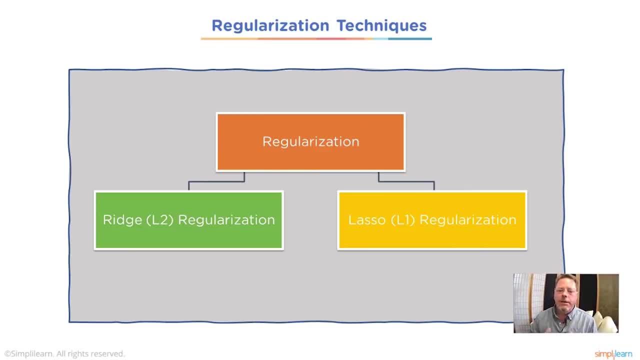 So what that means? uh, in this case, we're going to go ahead and take a look at a couple of different things. We're going to look at regularization, which we'll start with a linear model. We'll look at the ridge regularization and the lasso regularization. 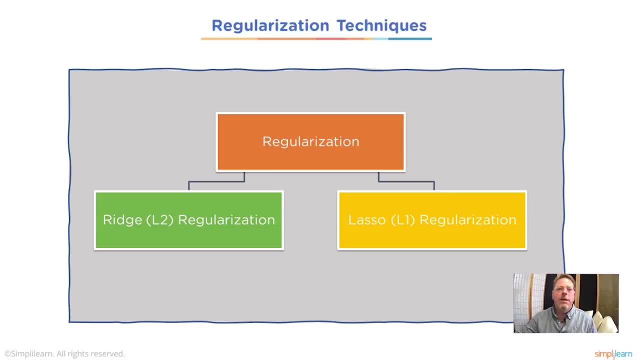 And these models are just like, uh, just like we did- the um, MLP, the multilayered positron, uh, linear regression models. And if you look at the linear regression model, you can see that if you had a linear regression model and you had a learning model, 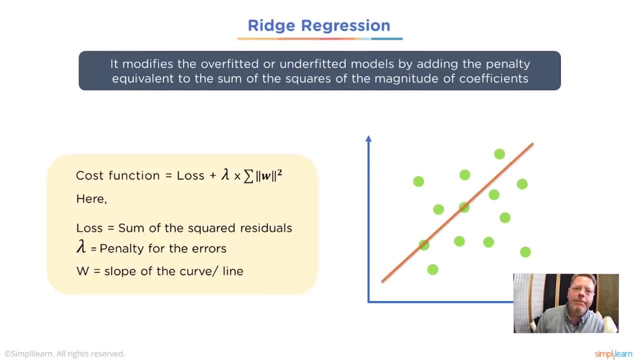 you could bring in the ridge module and you can bring in the lasso module. So when we talk about um ridge regression, it modifies the overfitted or underfitted models by adding the penalty equivalent to the sum of the squares of the magnitude of the coefficients. 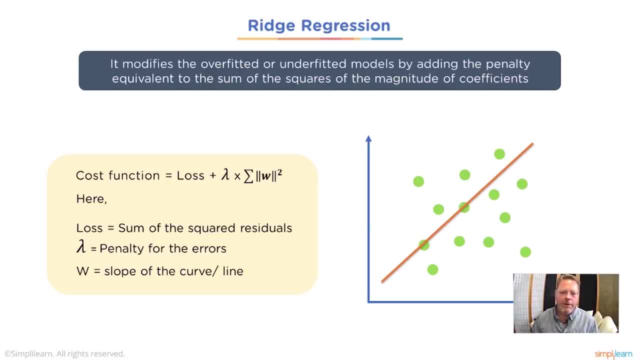 And so we have a cost function equals, loss equals on how you're doing it. Now remember we talked about error. whether we either square it or we absolute value it because it removes a plus or minus sign on there And there's reasons to do it either way, but it is more common to 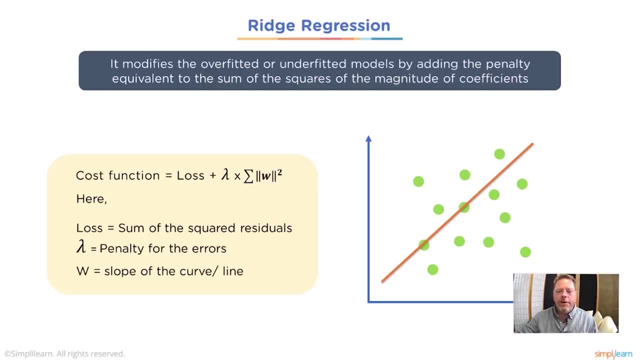 square the value And then we have our. in this case, the lambda is going to be the penalty for the errors. We've thrown in a Greek character for you just to confuse everybody: And W is the slope of the curve of the line. So we're going to look. 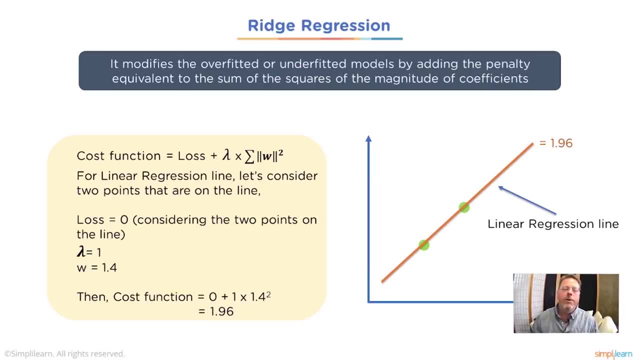 at this and we're going to draw a line. This is going to be like a linear regression model. So if you had in sklearn, you could import just a standard linear regression model. It would plot this line across. whatever data we're working on And we look at this and, of course, we're just extrapolating this. I 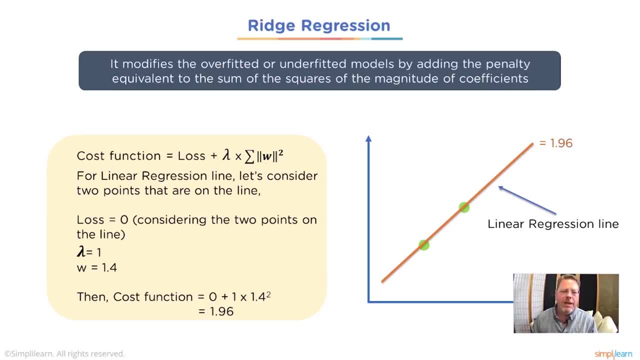 know they use some specific data but don't want to get into the actual domain. And so, for a linear regression line, let's consider two points that are on the line, And we'll go ahead and have a loss equals zero. Considering the two points on the line, we'll go and do lambda equals 1.. We'll 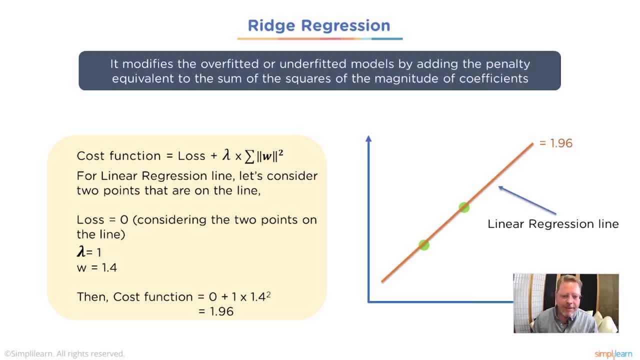 set, our W is going to be 1.4.. Then the cost function equals 0 plus 1 times 1.4 squared, which equals 1.96.. So really don't get caught up too much in the math on this, other than understanding that this is something that's very easy for a. 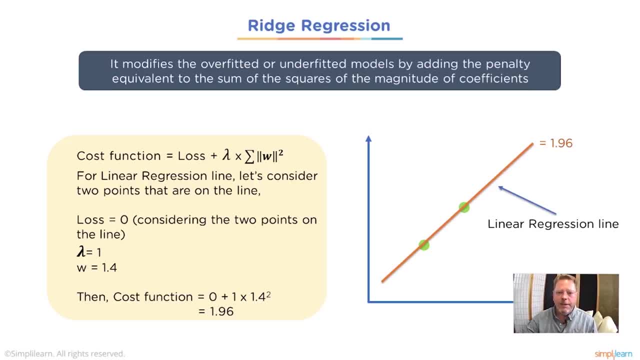 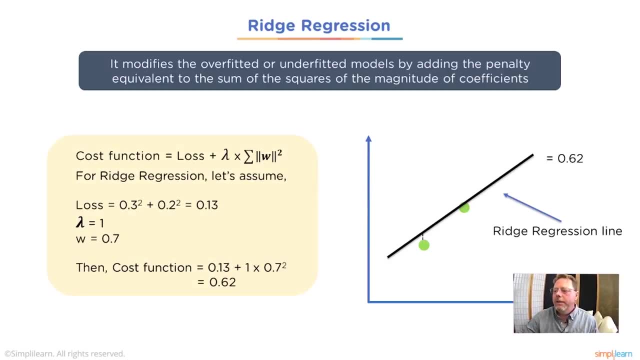 computer to calculate And if you ever see the loss plus the lambda times the sum of W squared. And then let's say we have a ridge regression line and it does this, We go ahead and plot it and we do the calculations on the data And for 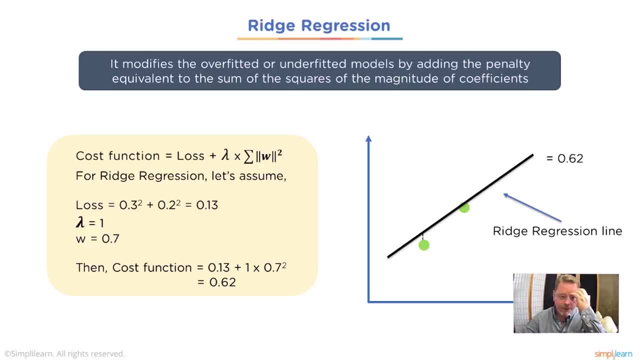 the ridge regression. let's assume a loss equals 0.3 squared plus 0.2 squared equals 0.13.. So when they put all the calculations through of the two points, we end up with a 0.62.. So we've now had a linear regression model. We now had a. 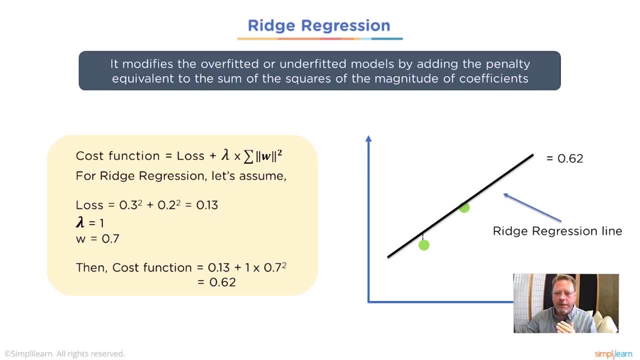 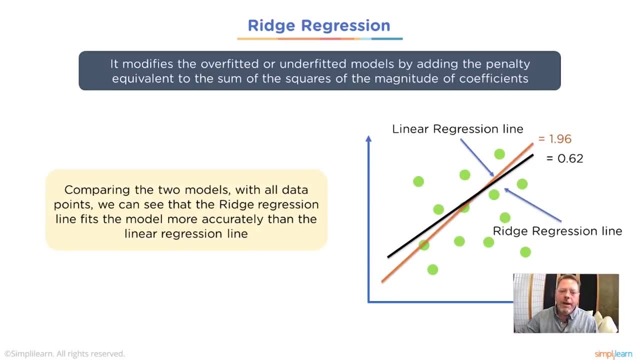 ridge regression model And the ridge regression model plots a little differently than the standard linear regression model And comparing the two models with all the data points, we can see that the ridge regression line fits the model more accurately than the linear regression line, And I find 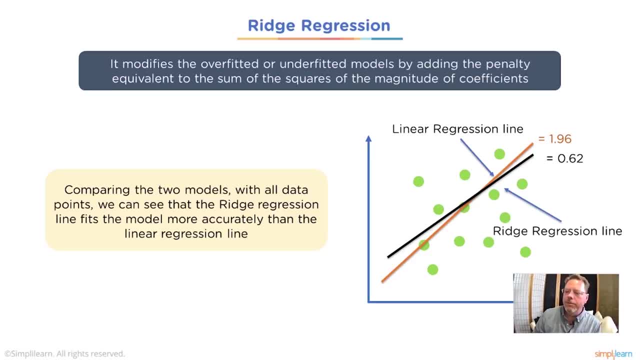 this true on a lot of data I work with. I'll end up using either the ridge regression model or the lasso Mars regression model for fitting, Especially dealing with a lot of like stock markets daily setup. They come out slightly better, You get a slightly better fit, And so we have our. 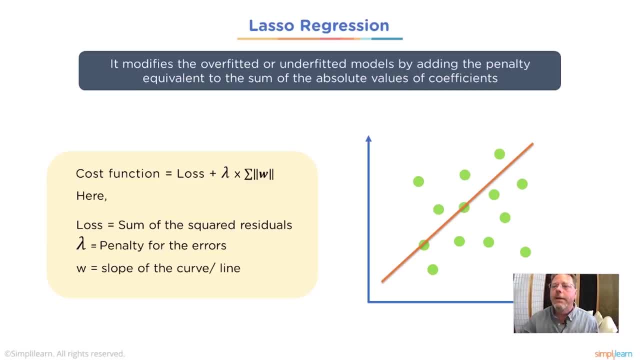 lasso- We just talked about lasso coming in here- And the cost function equals. instead of doing a squared, we're just going to do the absolute value, And so, if you remember, this is where ridge regression changes. Where's my ridge regression model? We're squaring the value here And if you look at this, we're. 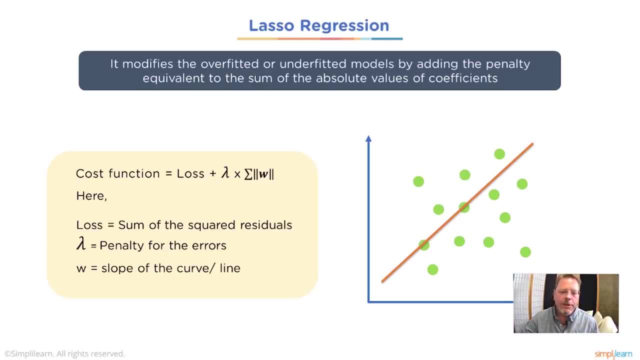 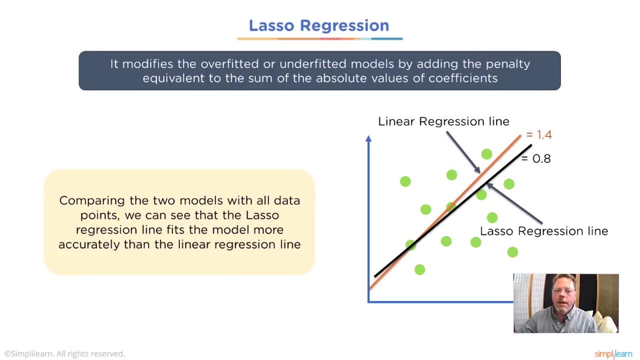 not squaring the value, We're just finding the absolute value on here, And so the loss of the squared individuals. And here is our lambda symbol again: Penalty for errors. And w equals the slope of the curve. And comparing the two models with all the data points, we can see that the lasso regression line fits. 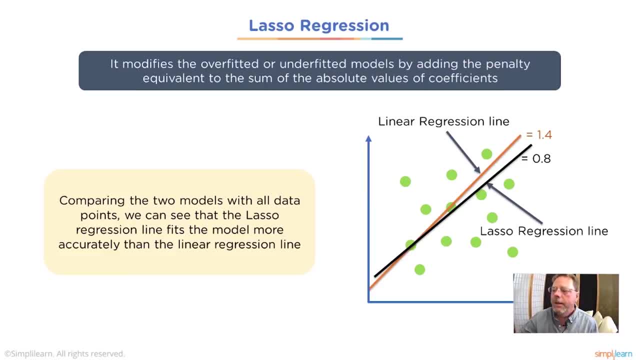 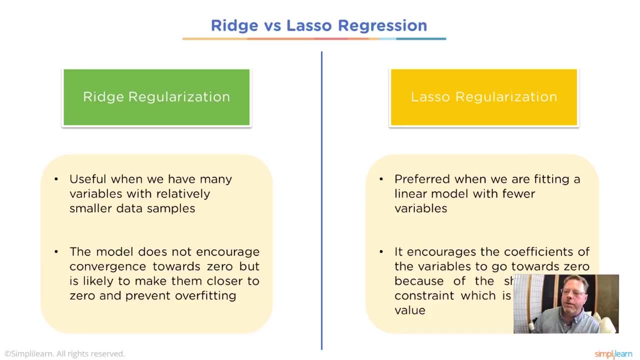 the model more accurately than the linear regression line, And this is like I said. I use these two models a lot. The ridge, and this is important, This is- this is kind of the meat of the matter- How do you know which one to use Some of? 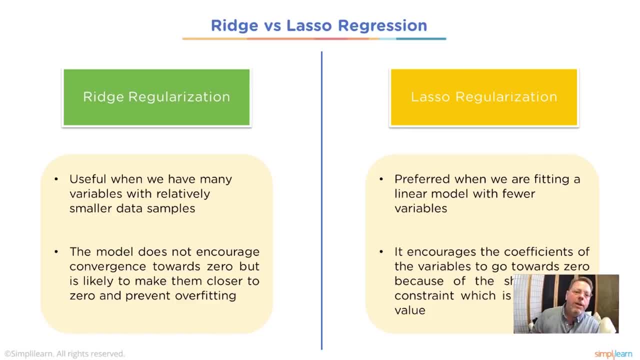 it is. you just do it a bunch of times and then you figure it out. Ridge regularization is useful when we have many variables with relatively smaller data samples. The model does not encourage convergence towards zero, but is likely to make them closer to zero and prevent overfitting The lasso. 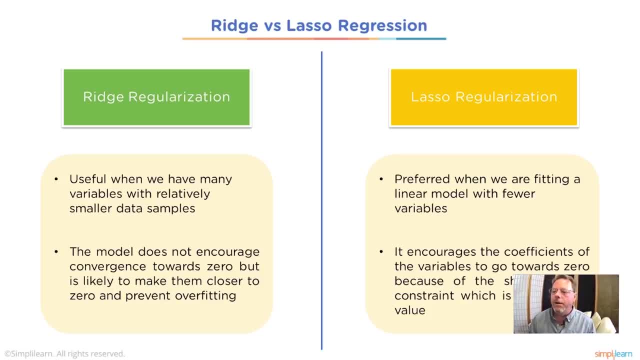 regularization model is preferred when we are fitting a linear model with fewer variables. So in the iris thing we had four or five variables as we measured the different leaf pieces. You might be doing the measurements on the cancer project which has 36 different variables. So as we get down to the iris with four, 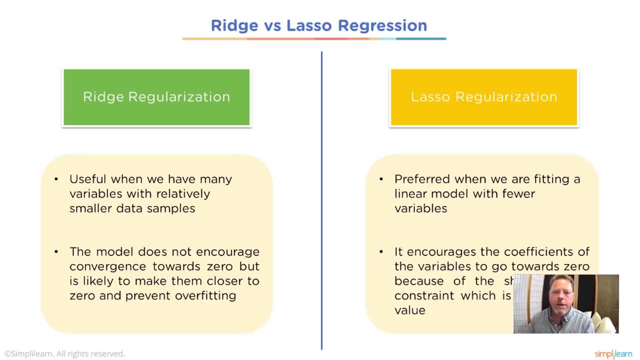 variables. lasso lar will probably work pretty good where you might use the ridge regularization with more model, with if you have something significantly larger, And it encourages the coefficients of the variables to go towards zero because of the shape of the constraint, which is an absolute value, And with any of this, 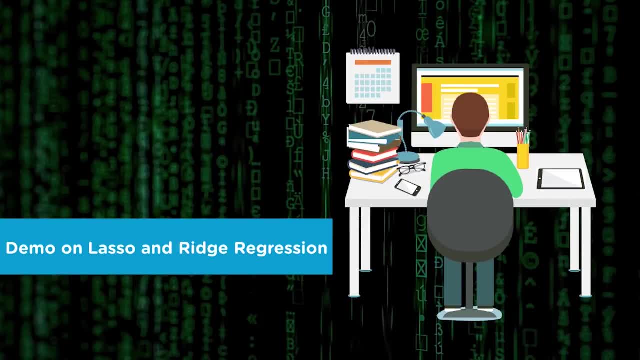 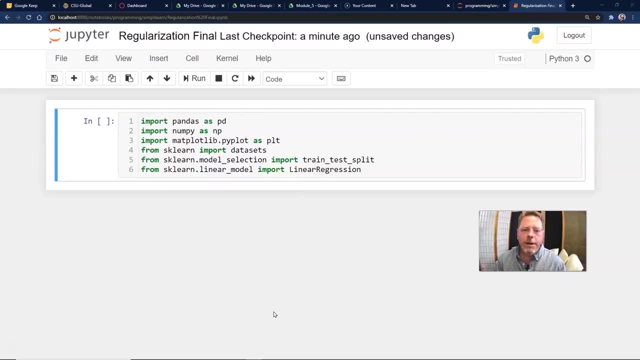 we want to go ahead and do a demo and lasso and ridge regression. So let's take a look and see what that looks like in our code and bring up our Jupyter notebook. We'll start with our imports: Pandas as PD import. 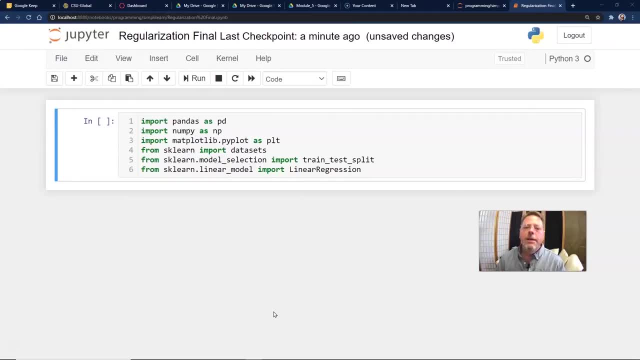 numpy as Np. Import matplotlib library as PLT. sklearn- we're going to import our data sets. It's kind of more generic. We usually just import one data set instead of all of them. but you know quick and dirty when you're putting some of these together. 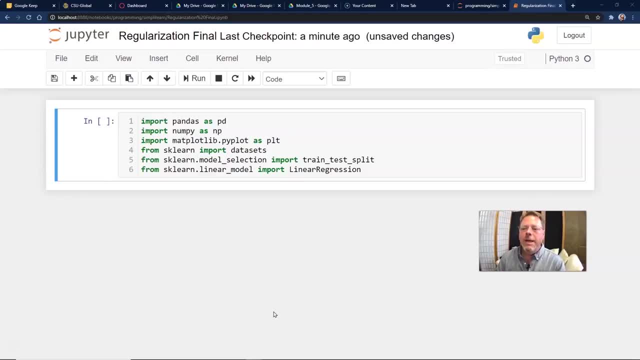 we have our sklearn model selection. we're going to import our train test split for splitting our data up, and then we'll bring in our linear regression model and we'll go ahead and run these just to load them up and then load our data set. we were just talking about that. you could just have. 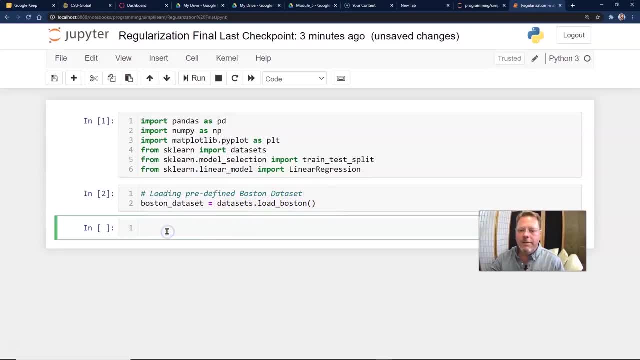 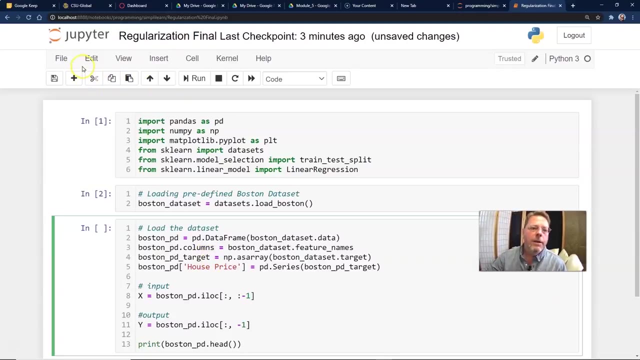 imported the load boston and boston data set in there, instead of loading all the data sets and then, once we've loaded our data set, we want to go ahead and take a look at that data and see what we got here. let me just go ahead and pop that down there and go ahead and run it. 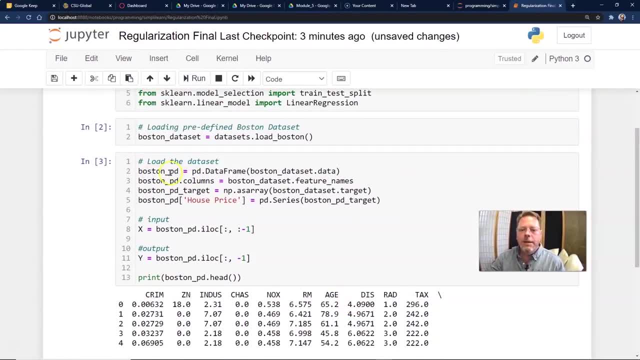 and so we've gone ahead and taken our boston data. we're going to look, we put it into our pandas data frame, the boston data set and then the boston columns. so we want to see what's going on with them. we have our target, we have the house price. 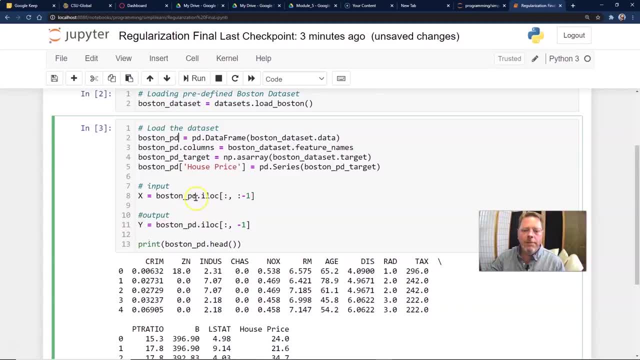 etc. and so our x equals boston i location. now remember, in pandas, the new updates to pandas, they want i location if you're going to pull data. we used to be able to leave this off, but it does something different. it creates a slice versus a direct setup, so make sure you're using that. 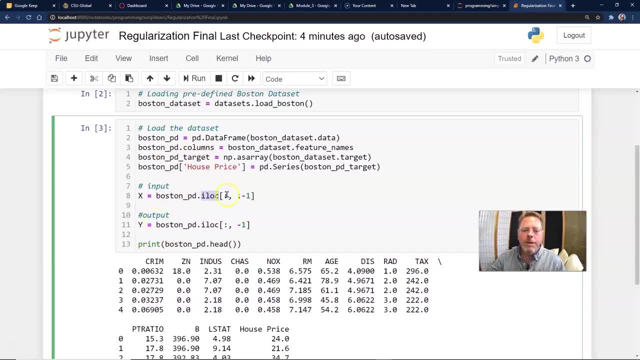 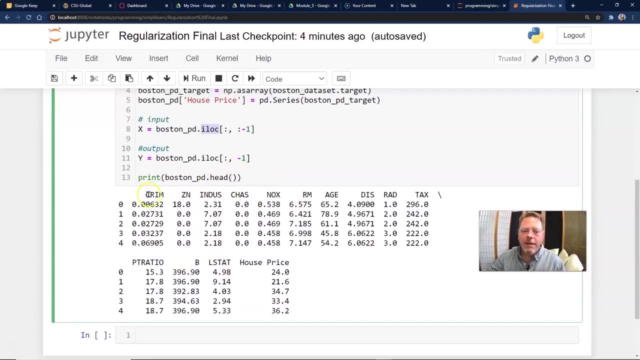 i location and the i the output. so this is all just bringing our data together and we can see here if we do we print the boston data set. and we can see here if we do we print the boston pandas head. we can see here all of our different aspects we're looking for. 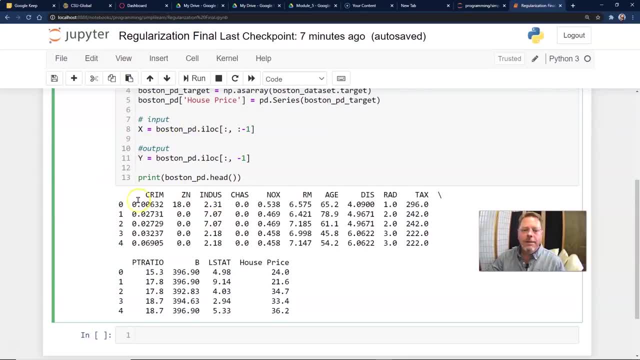 and if you're following the x and the y, the x is everything except for the last column where y is, uh, all the it's. that's what this means: all the rows except for the last column. and then y is all the rows but just the last column. so y is our house price and the 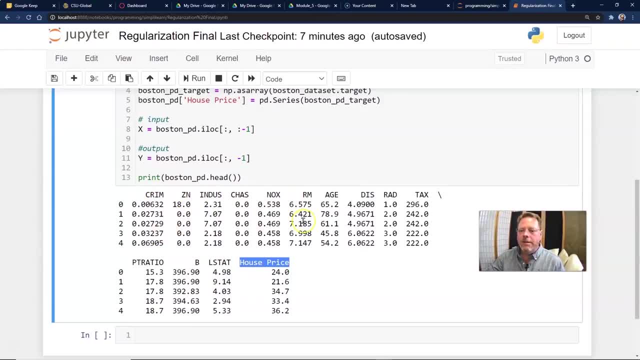 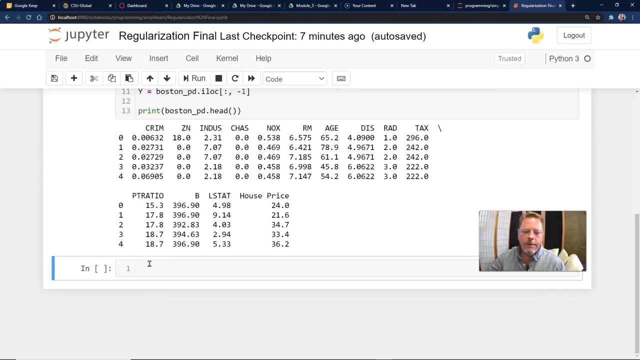 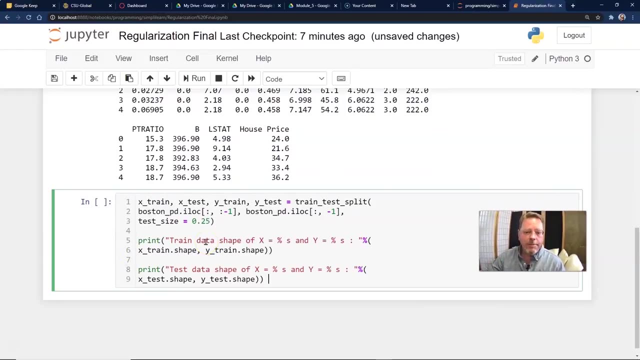 next row is the cost of product. so that's everything we have on the boston boston and then all the other options we have is the crime, zn industry, chas, knox and all these other different statistics they've collected for house sales in boston. 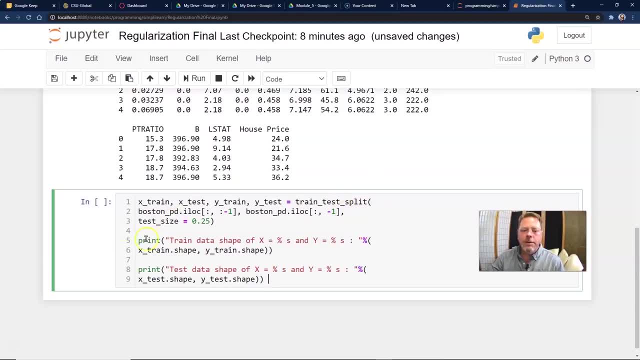 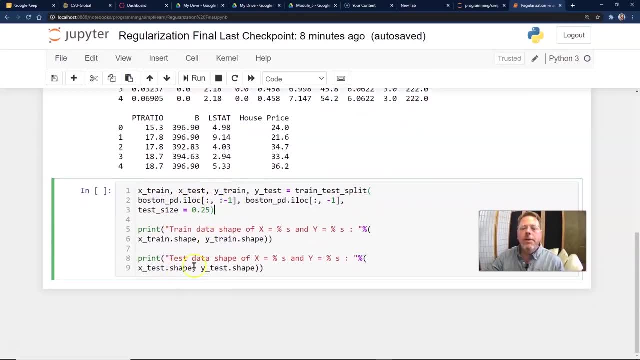 there we go. whoops, control our boston. you could have easily used the x and y on here as opposed to boston i location, and we'll create our test size. we're going to take 25 of the data and put it in as a test. 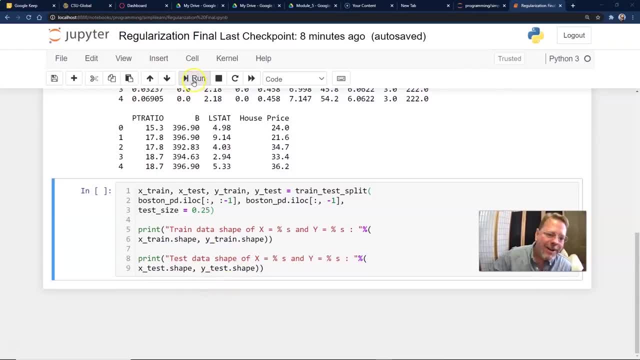 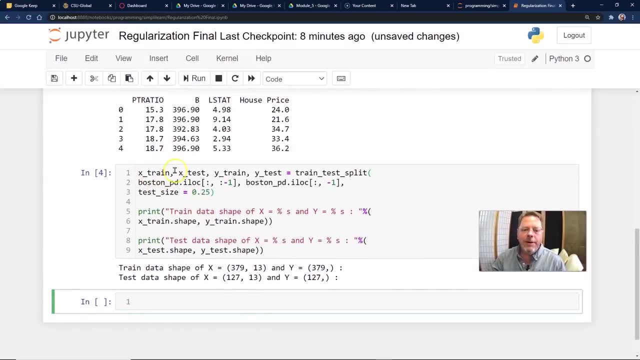 and then we'll go ahead and run. this need an extra drink there. so we have our train and test. and then, of course, the print, the train data shape. i love doing this kind of thing. whenever i'm working with this data print out the shape, make sure everything looks correct so that we have 127 by 13 and 127 by 1, 379 by 13. 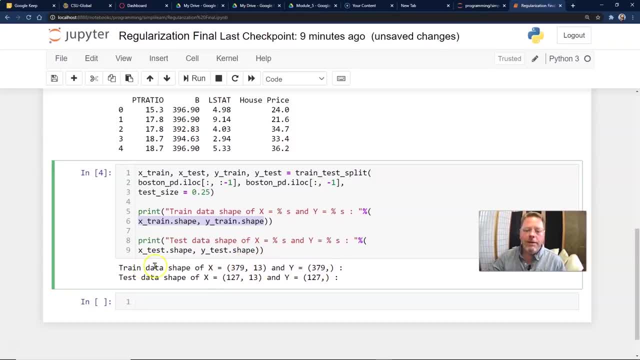 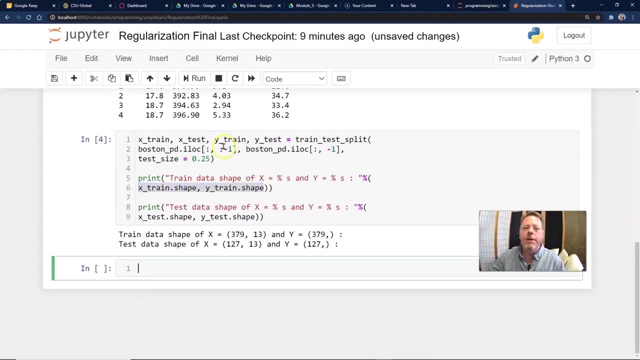 they should match. and if they're, if the the data sets are not quite matching, then you know something's wrong and you're going to get all those errors. i don't know how many times i've gone through here and it's dropped a row on one of them and not on the other, or something. 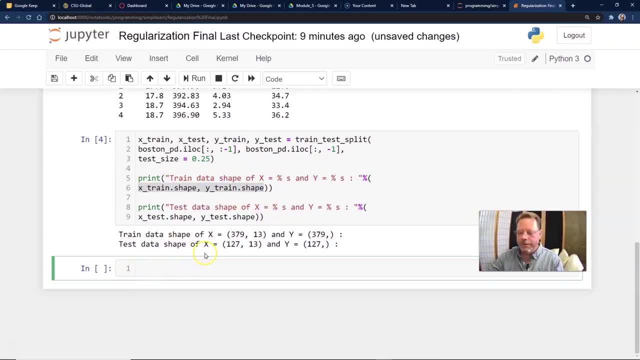 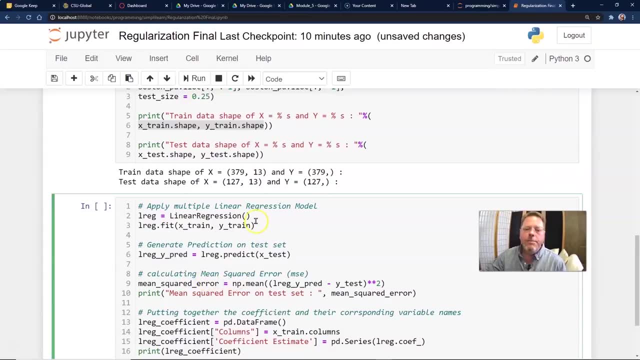 weird has happened when i'm cleaning the data. this is pretty straightforward and simple because the data comes in a nice pre-package, is all clean for you, so let's go ahead and apply. apply the multiple linear regression model and we'll call this lreg- lreg, linear regression- and we're going. 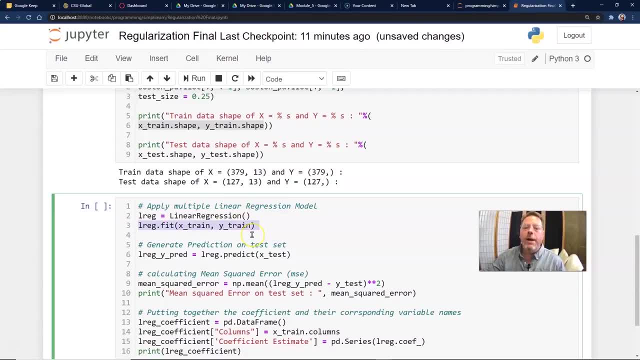 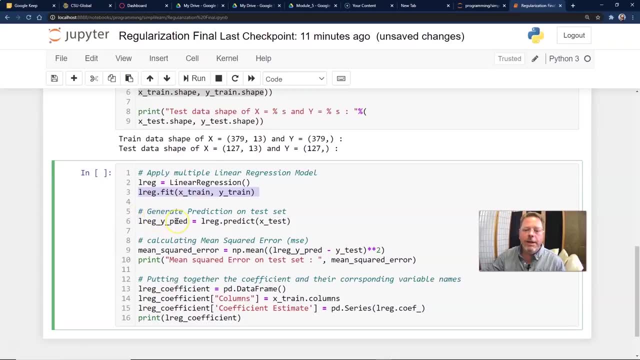 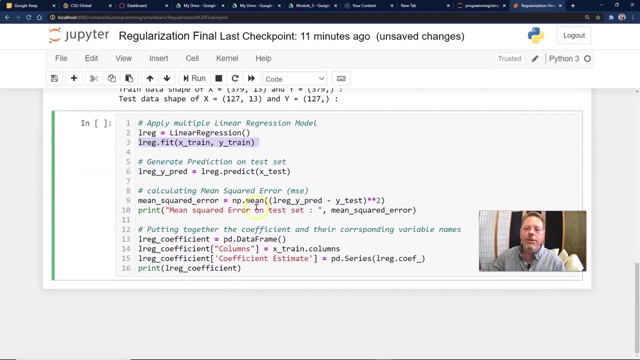 to go ahead and fit that linear regression model to x train and y train, then we'll generate the prediction on the test set. so here we go. here's our lreg y predict with our x test going into the prediction, and let's calculate that mean square error, mse. i told you you'll see, mse used a lot. 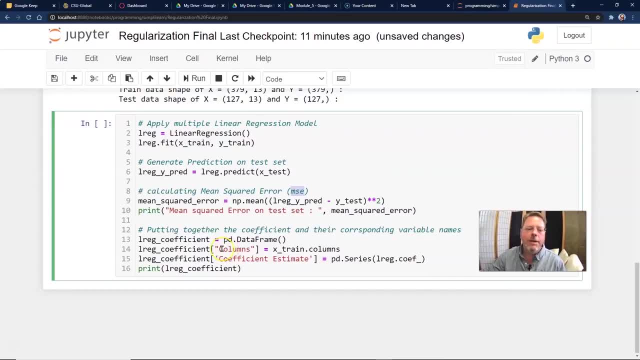 people use it in variables and things like that. it's pretty common and we get our mean squared error equals. this is just the basic formula. we've already been talking about what's the difference squared? and then we look for the average of that. we'll go ahead and just run this. 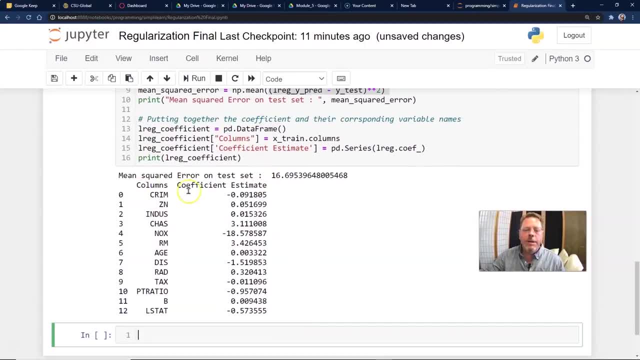 code and you can see when we get through the end of this. we have our mean square error on test, we have our total and then we have each column coming down and at this point, unless you really know the data you're working with, it's not going to mean a whole. 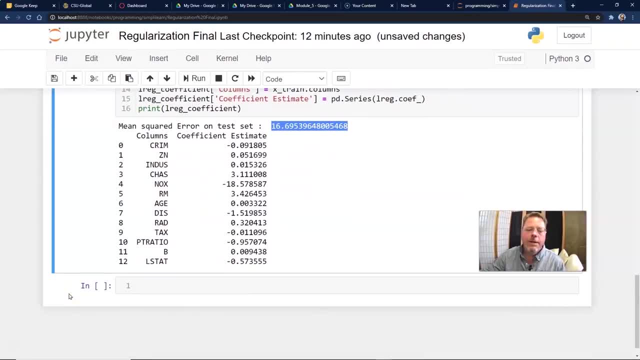 lot. so if it's in your domain, you might be know what you're looking at when you see these kinds of numbers coming up. but if it's not, it's just a bunch of numbers and that's okay. at least that's okay for this demo. sorry, sorry, sorry. 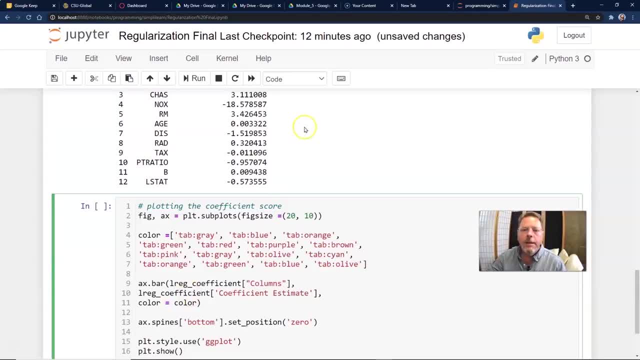 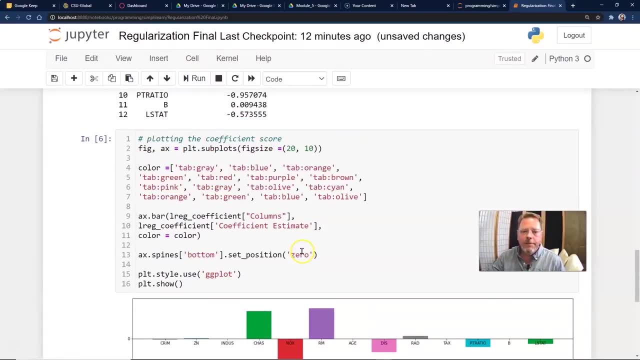 And then we're going to go ahead and plot these so we can see what's going on. And this is always kind of fun. It's always nice to have a nice visual of what you're looking at And you can see. here we plot the coefficient scores on here. 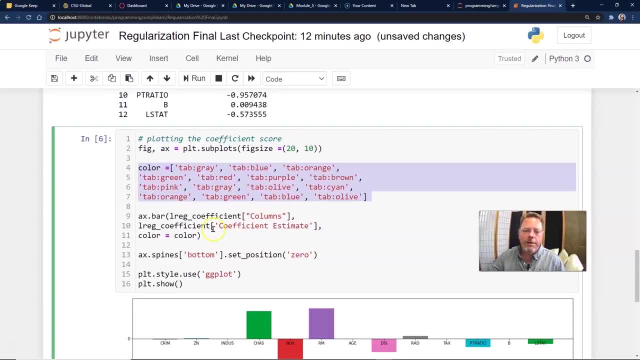 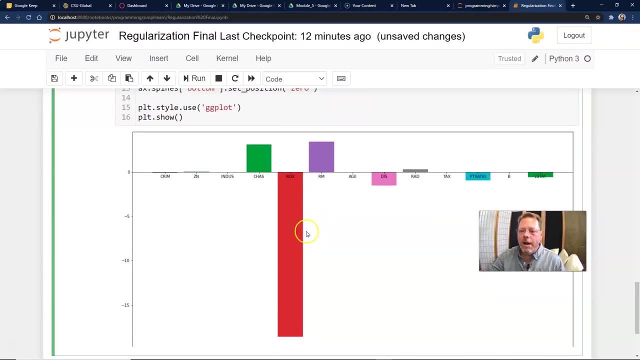 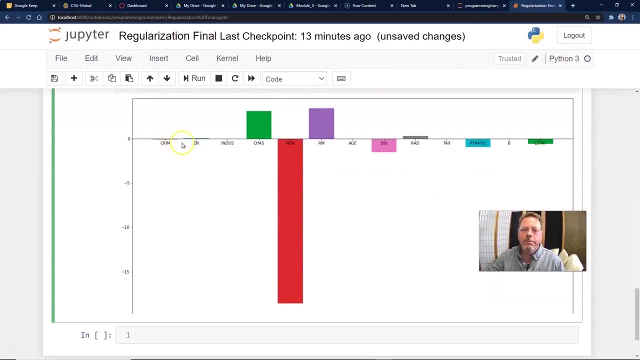 And the guys in the back did a great job putting some pretty colors together, making it look nice and setting up the columns. You can see here your NOX has just a huge coefficient. When I look at a table like this, I look for what has very little different coefficients. 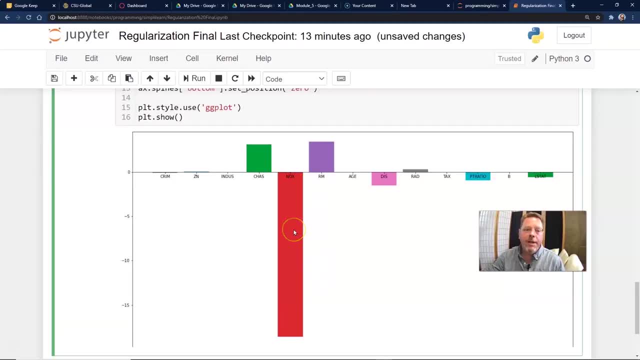 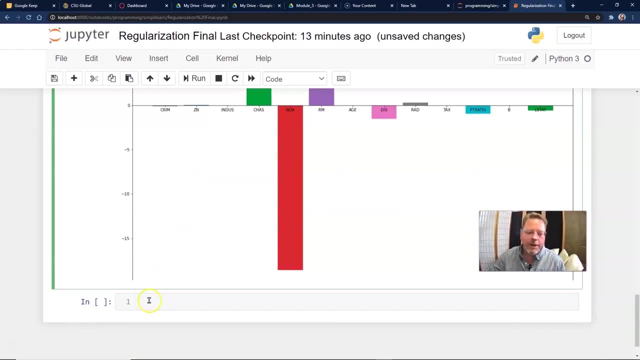 They're not using a huge change and what has huge changes, And that flags you for all kinds of things as you're working with the data, But it depends so much on the domain you're working with. These are great things, though, as just a quick look to see what's going on with your data. 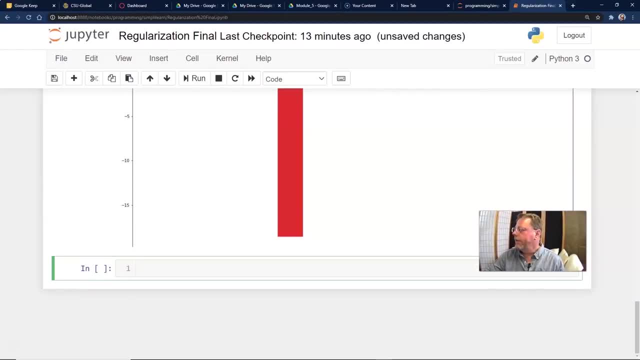 and what you're looking for. And of course, once we look at this now, our motive is to reduce the coefficient score. So now we want to take these and bring them down as much as we can, And for that we're going to work with the ridge regression on here. 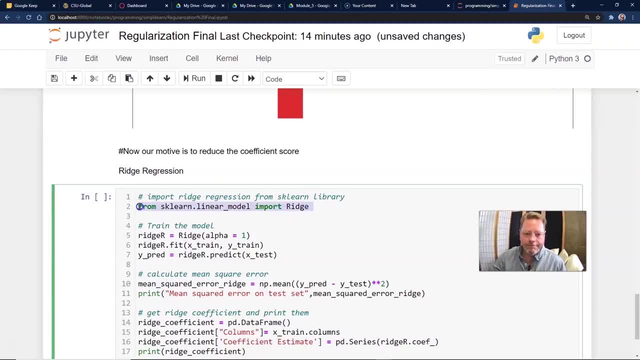 So let's start by going ahead, and we're going to import our ridge model, the ridge regression, from the SKLearn library or the Scikit And we're going to go ahead and train the model. So here's our ridge: R equals alpha equals 1.. 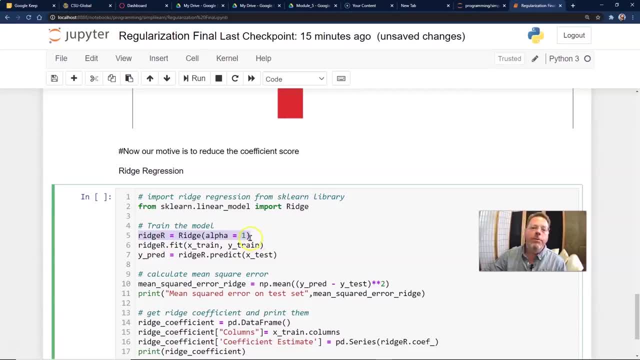 And I mentioned that earlier When I work with the ridge model. see: alpha equals 1.. If you set alpha equal to 0, that's a standard linear regression model. So you have alpha equals 1,, 2,, 3,, 4, and you usually use 1,, 2, or 3,, 4 in a standard integer on there. 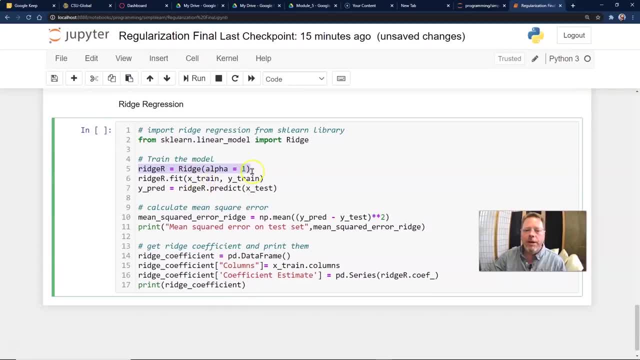 And we'll go ahead and fit the ridge model on there with our x-train and our y-train data, Generate a prediction for that for our x-test, And we'll calculate the mean square error just like we did before. This should all look familiar. 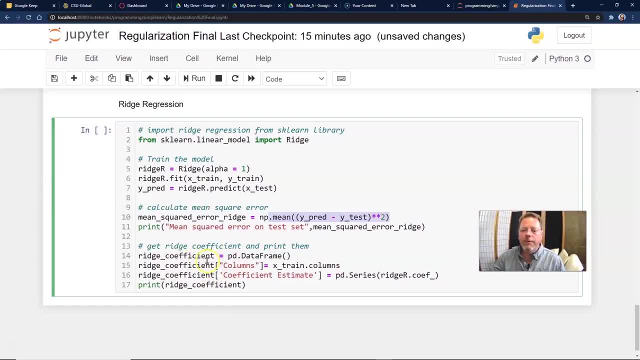 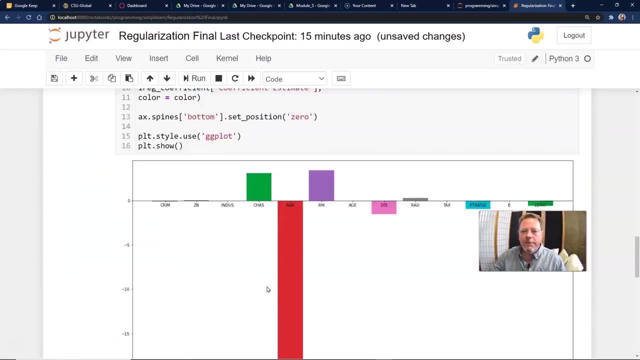 And we'll go ahead and print that out And we'll look at the ridge And we'll look at the coefficients for our data and see what that looks like. Now, if I jump up and down between these two, you'll get a headache. 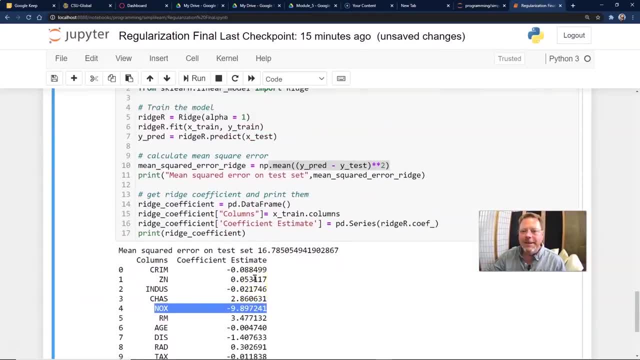 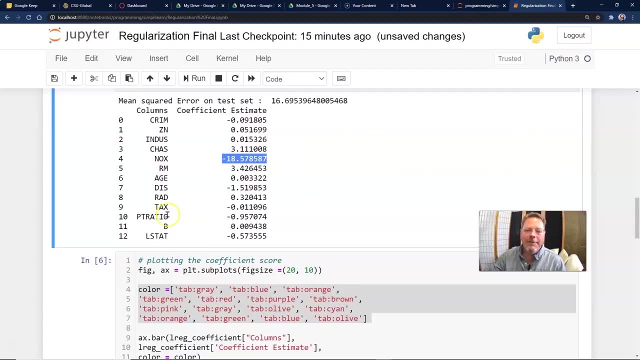 You'll still see the NOX value. Let's just look at the NOX, because that was the biggest value. It's a minus 9 here And if we go back up here, the NOX value is a minus 18.. So right off the bat I'm seeing a huge change in the biggest coefficient. 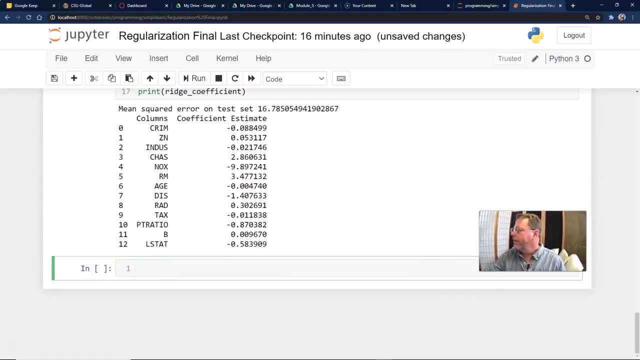 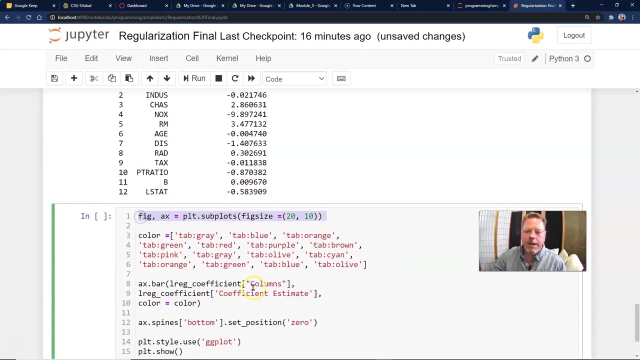 There. So if we're going to do that nice setup, we want to go ahead and just print it and see what that looks like. Here we go And we've set up our plots, subplots, And again, the team put together some nice colors, so it makes it look good. 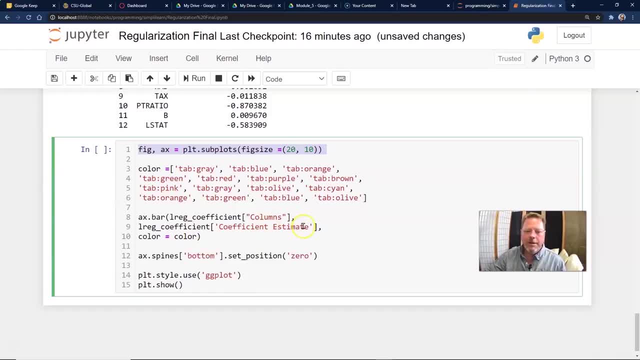 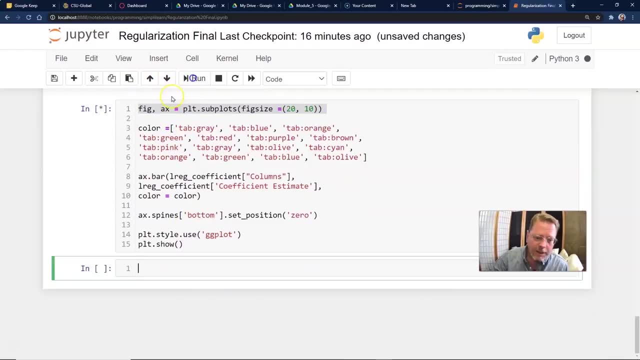 We're doing an x-bar based on the columns and our L-regress coefficients: Color equals color X, spine bottom and so forth. So it just puts together a nice little graph And you're starting to see one when you compare this. 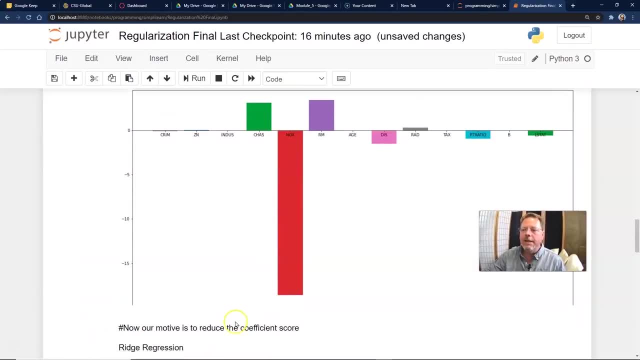 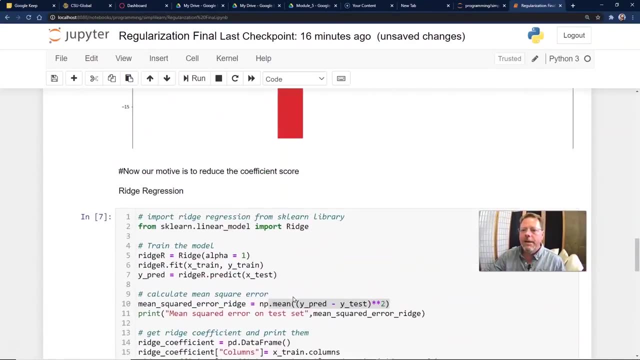 if you put it on the same graph as this one up here. this is up here at minus 18.. This is at minus 9.. And so this graph is half the size of the graph above. The same thing with these values here. 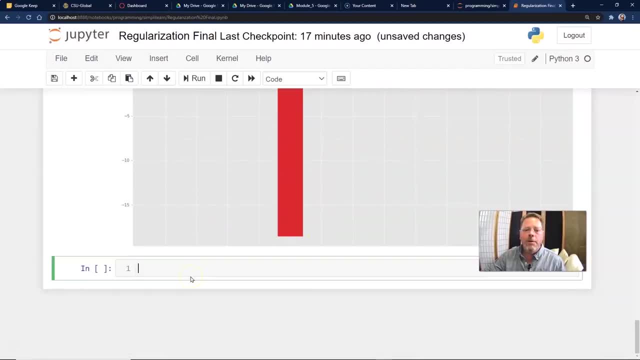 They might look the same, but they're actually all almost half the value on here. And then, finally, you can do the same thing for the lasso regression. This will all look very similar as far as what we worked on before, And I'm just going to go ahead and print that on here and run it.